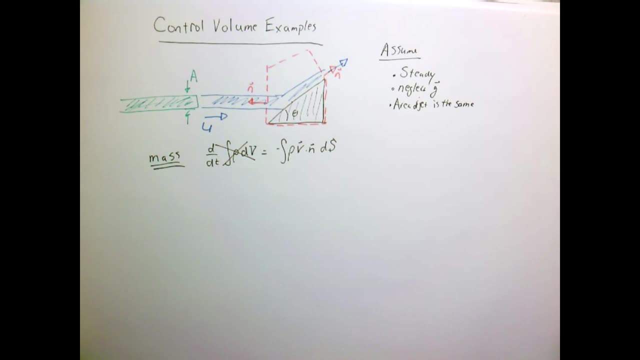 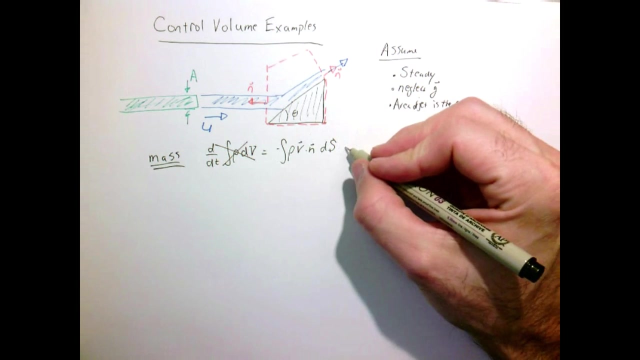 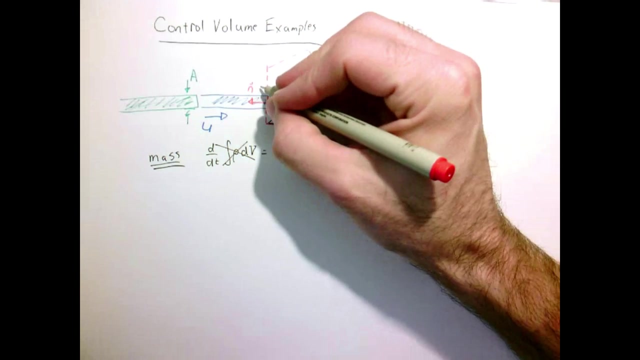 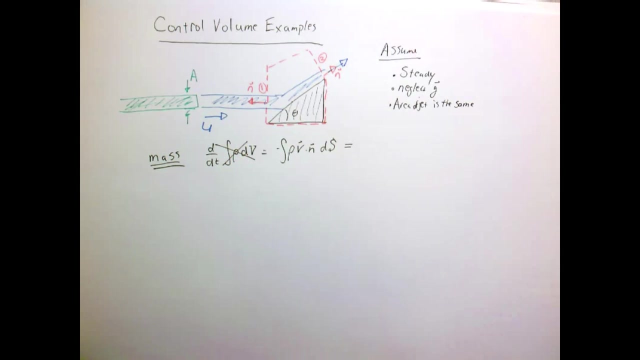 I can get rid of that term, And since this side is zero, I can basically get rid of the minus sign, And so I just have rho v dot n on my boundaries, So I really have two places to worry about it. I'll label them one and two, So I have flow coming in here and going out there. 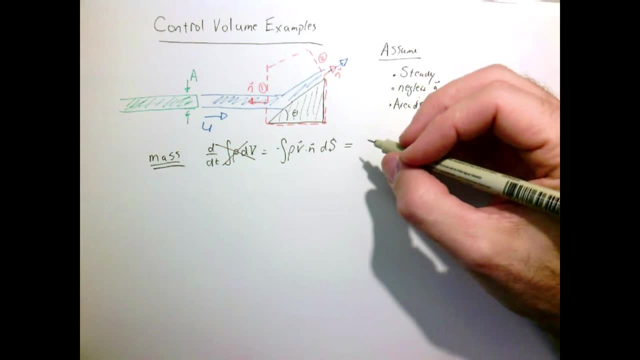 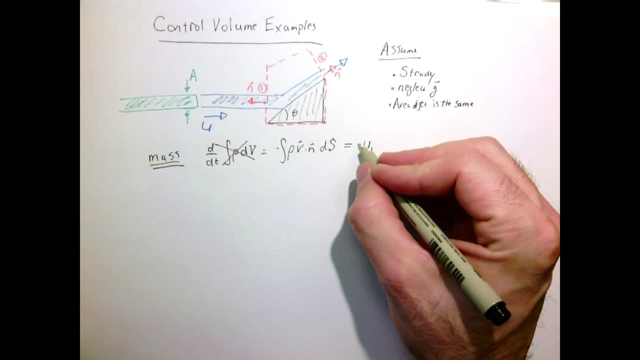 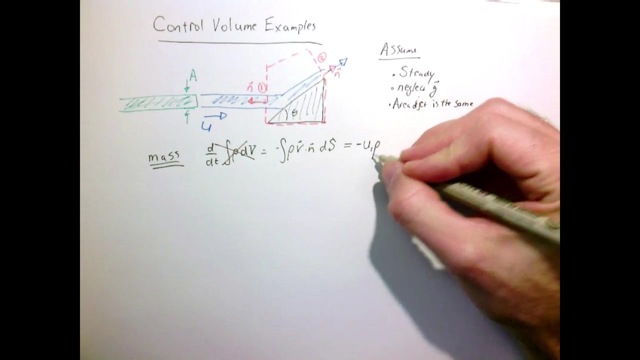 Now, if we're going to assume that the velocity coming out is uniform, then the velocity at one dotted with the normal vector will be negative. since velocity is in this way and the normal vector is outward, We're going to have the density of the fluid, rho and we're going to have the area. 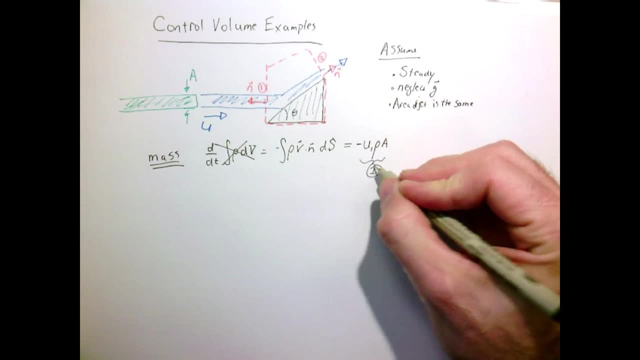 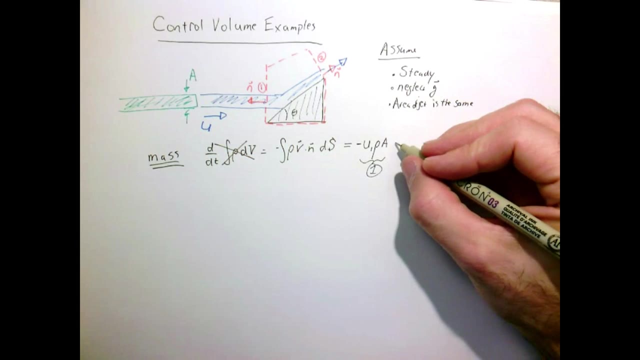 of the jet a. So that's at surface one. At surface two the velocity is aligned with the normal vector. so I have plus u. at location two I have the density of the fluid and we're assuming the area of the jet is the same. So a1 equals a2 is equal to a times a and that equals to zero, because it's. 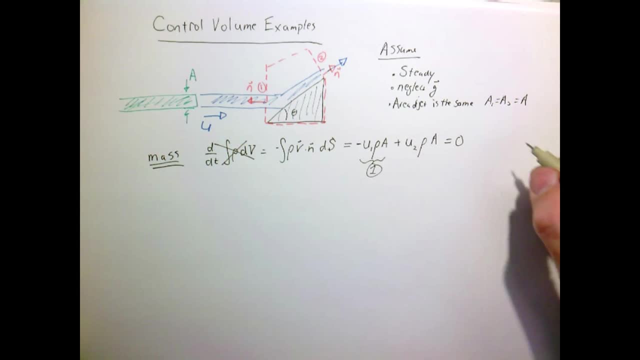 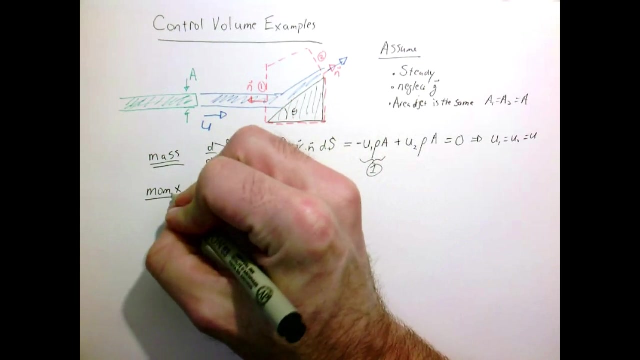 steady. So now we see the density and the area cancel and this tells us. what we probably could have guessed was that u1 equals u2 is equal to just the velocity of the water coming out of the hose. Now let's consider momentum in the x direction. 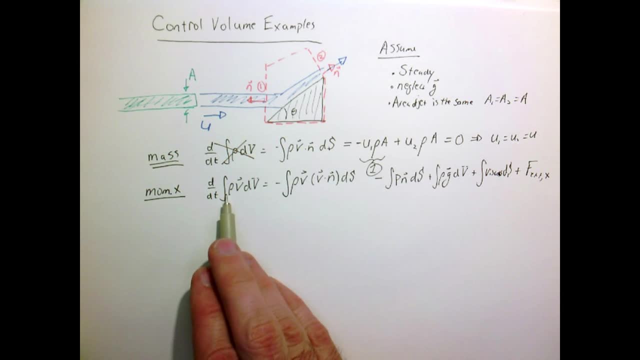 So we have several terms here. We have the time rate of the change of the momentum in the control volume, the flux of momentum in and out, the pressure, gravity, viscous stresses and our external force. Since I drew my control volume, 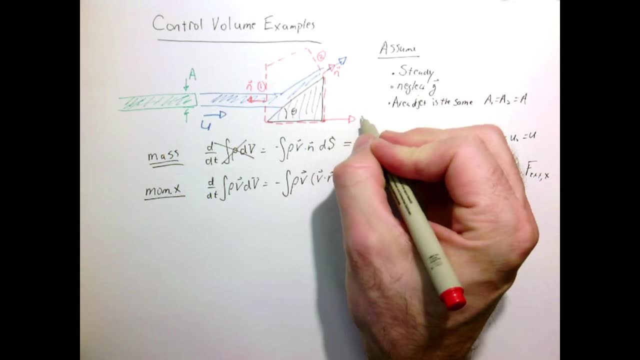 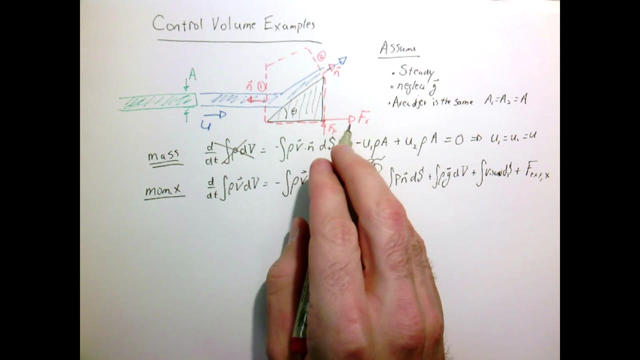 to sort of enclose the block. we need to imagine that there must be some external force which has an x and a y component that's holding the block in place. And so my external force I'm going to draw with the assumption that it's positive, so I can just conclude it's a positive number here. 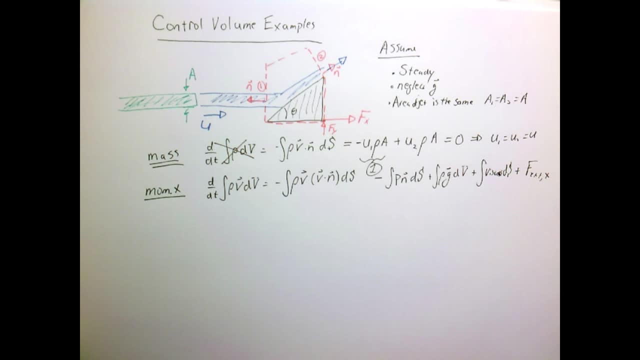 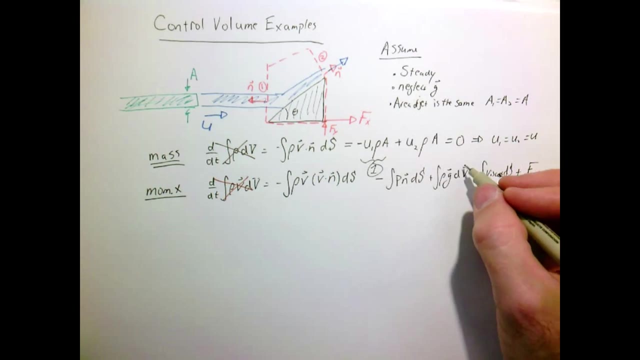 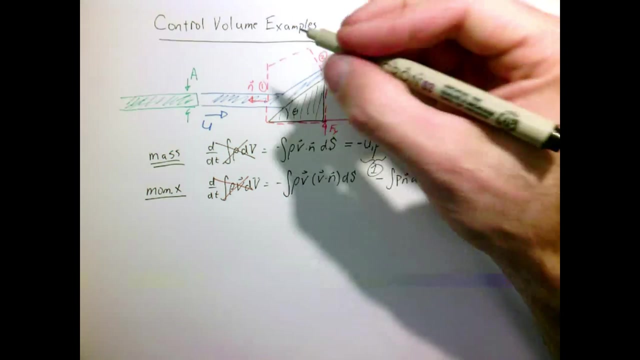 and the sign will work out in the end. Okay, so let's look at our assumptions again. So by steady flow I can get rid of that term, By neglecting gravity I can get rid of that term. And then also, if we just think a little bit physically here, the pressure. 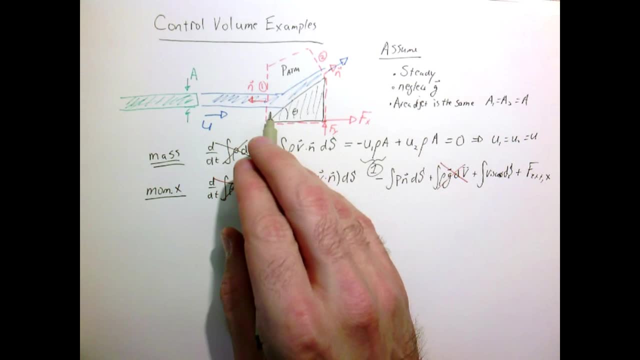 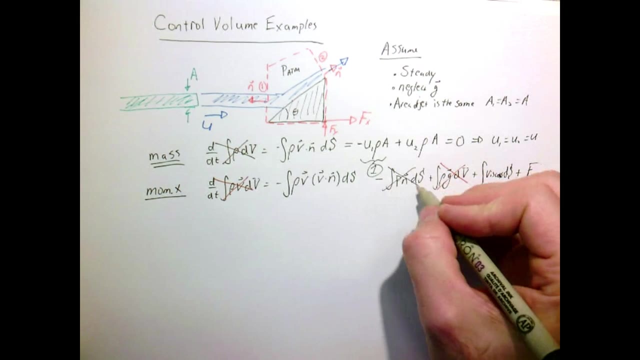 this is just the jet in air, it's just the atmospheric pressure. it's the atmospheric pressure here, it's kind of the atmospheric pressure everywhere. So there's no reason for us to build up pressure inside the jet. so there's no net pressure force, it's acting on. 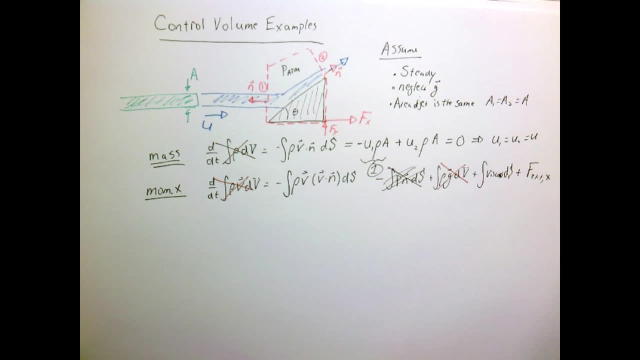 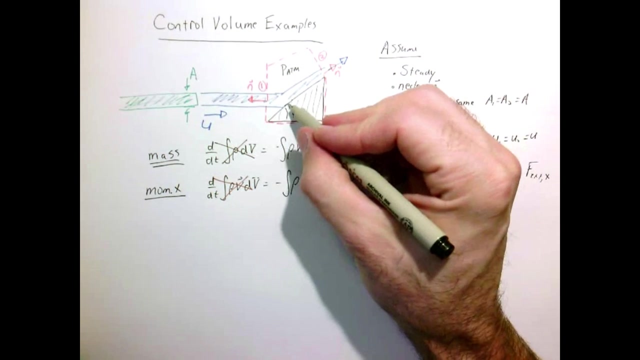 it's just atmosphere pushing on it everywhere. So in the end we have flux of momentum, external force and the viscous stresses. However, these are the viscous stresses of the boundary ds. So we know that, all the viscous stresses, if there were any to worry about. 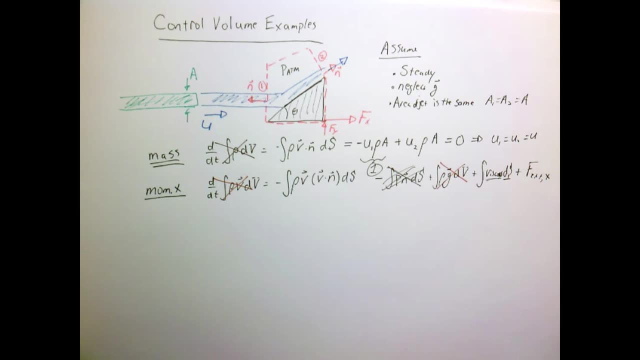 would be located along this surface, And so what I'm going to do is sort of say: let's cut our boundary here and here, and so in that case there would be actually no viscous stresses at this location and this location, So along the surface then the viscous stresses are zero because we're 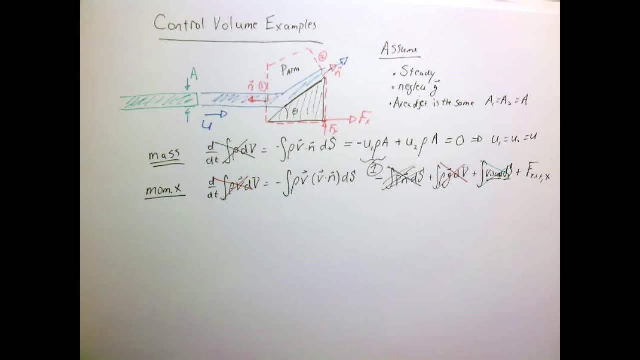 just looking here and here, And so in this case, any viscous stresses would be wrapped up into the external force. Now, this is a little bit subtle, so we'll actually deal with this in the next problem, but let's just move forward saying there's no viscous stresses on the surface. 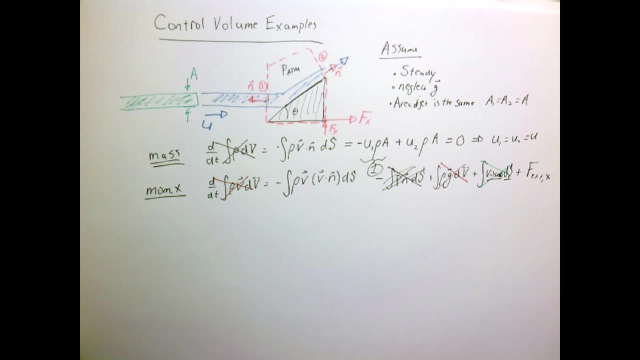 of our control volume. Okay, so now let's evaluate all the terms. We have to be a little bit careful with the sign. There's a negative sign here. This rho v is a vector, so we have to worry about the sign there. 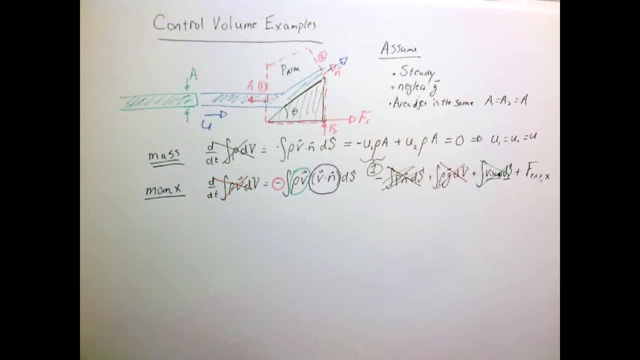 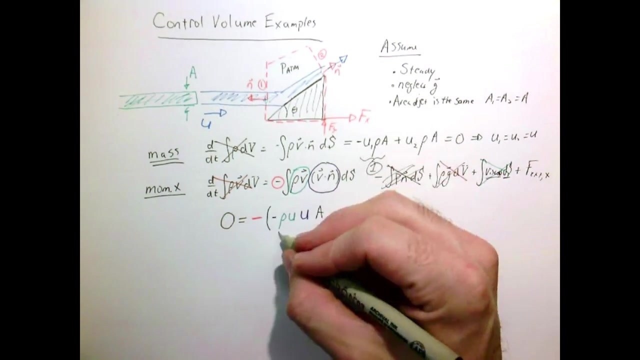 And v dot n can have a negative sign here And v dot n can have a negative sign here. So we have kind of three negative signs we always have to keep in mind. So our equation then is that zero is equal, So on surface one rho u is the momentum coming in, v dot n is just u, with a negative sign because 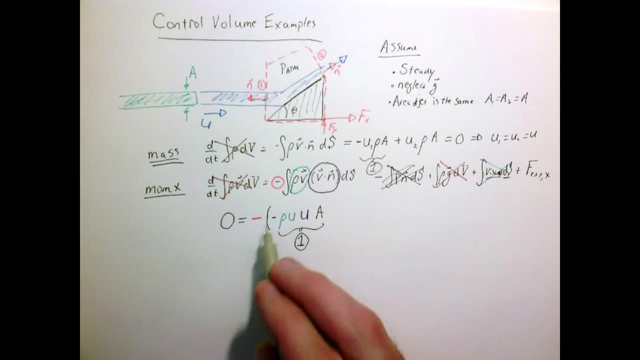 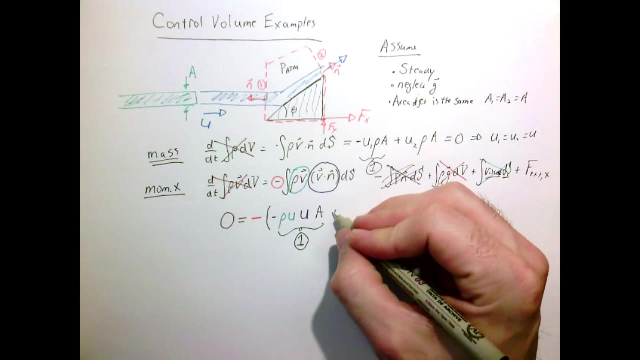 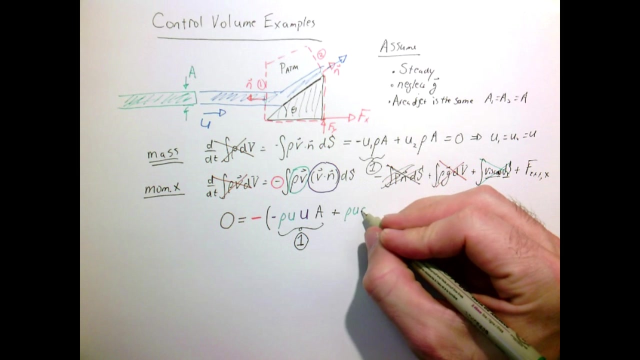 the normal vector points out the velocity's in, so that's negative. And then I have ds for just assuming it's constant over the area of the jet. so it's just multiplied by a At surface two, rho v right v is a vector, so it's rho u cosine theta. 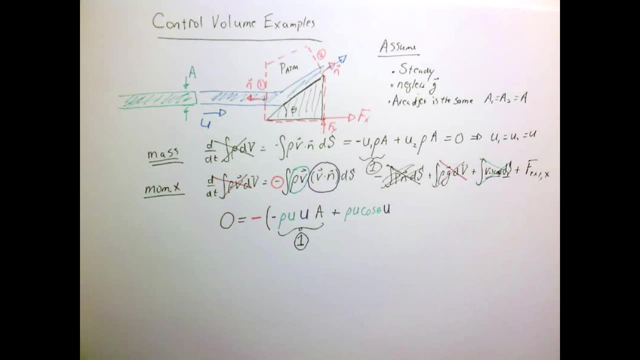 v dot n. in this case they're aligned. so it's just u times the area of the jet, And that's equal to two. So we have a vector plus the external force in the x direction. So what does that imply then? That implies that the external force f of x is rho u squared a. 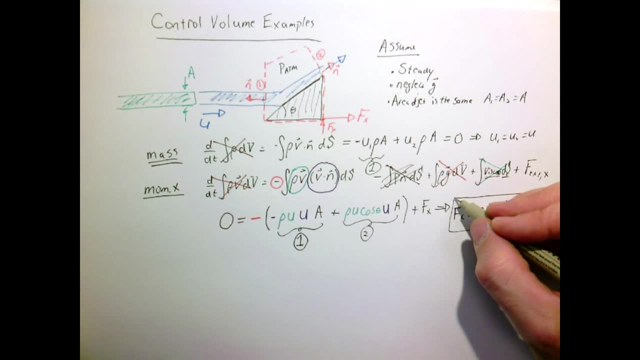 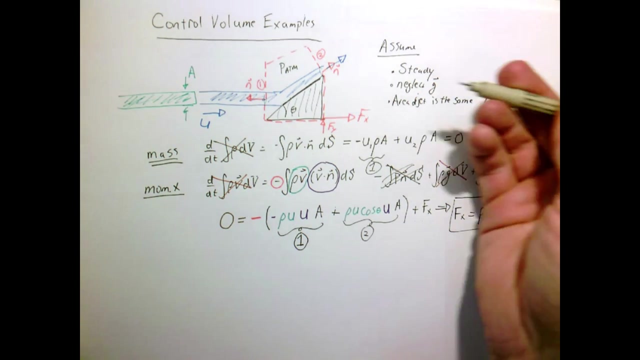 cosine theta minus one. that makes sense because cosine theta will be less than one, so this will always be a negative number, so our force will have to hold the block in this direction. If the angle were zero, then this would be zero, so there'd be no force. If the angle were 90 degrees, the force would be maximized and 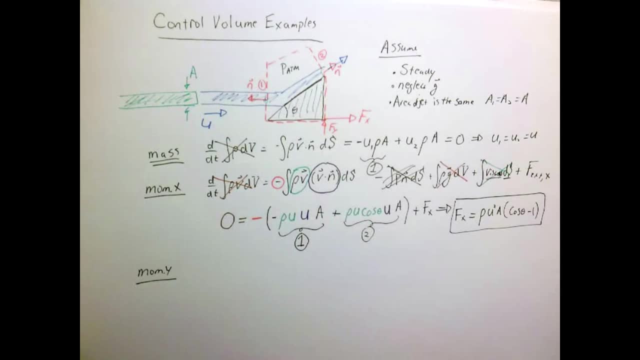 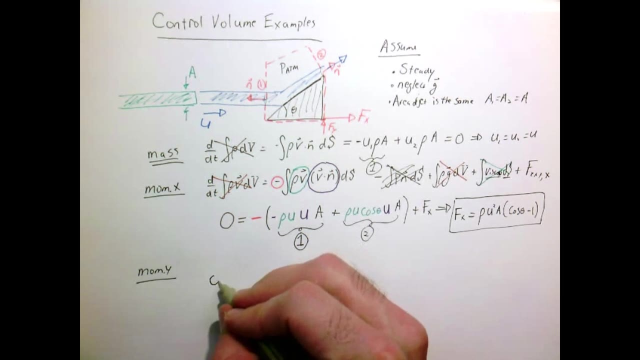 negative. Now let's consider the y momentum, and again we can just look at this expression up here. so we have zero, because it's steady is equal to. again we have our negative sine. On surface one there's no vertical velocity, so rho v is zero. On surface two, rho v is rho. 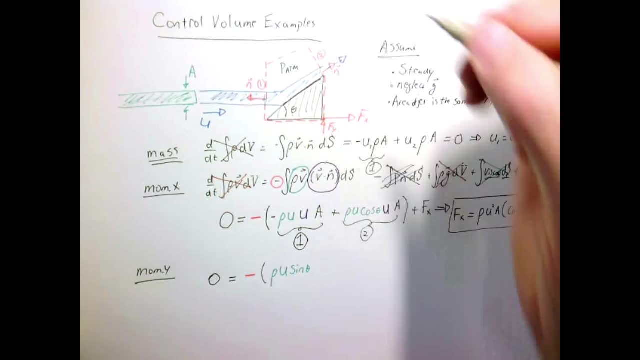 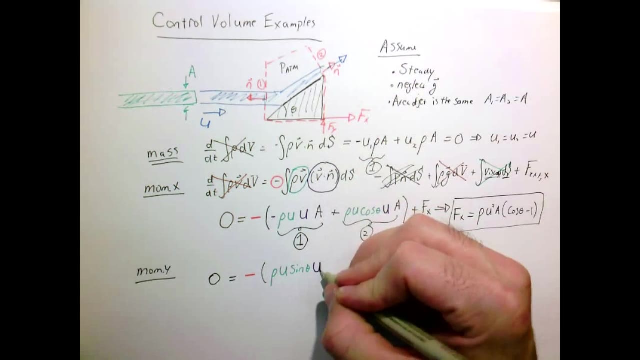 u sine of theta, because that's the vertical velocity there and the flux out of it v dot n is aligned and positive. so it's just u plus v dot n Times the area plus the external force in y. So that implies then that the force in y is rho? u. 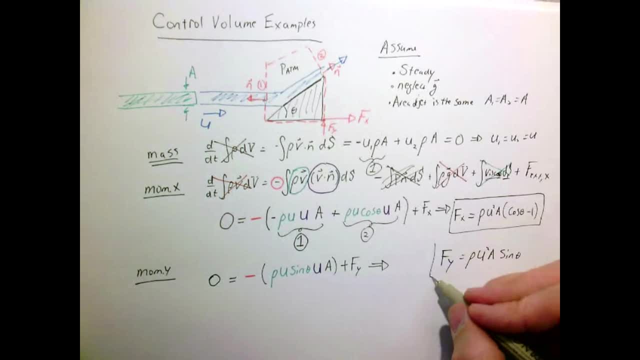 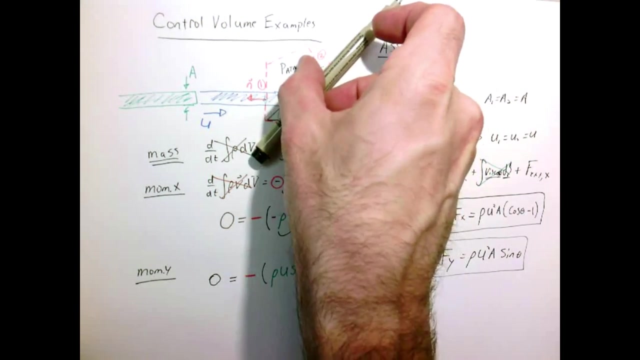 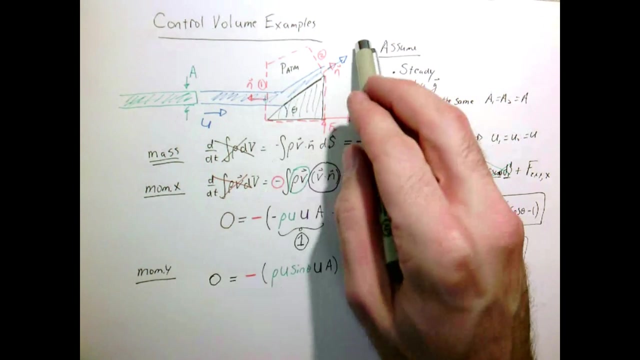 squared, a sine of theta, and it's positive, so it's a force upwards. So when the angle is zero, there's no force holding the block upwards, and as we change the angle here it gets steeper and steeper. Then the force pushing the block down gets stronger and stronger. and that's assuming that all the flow goes in and out and up. 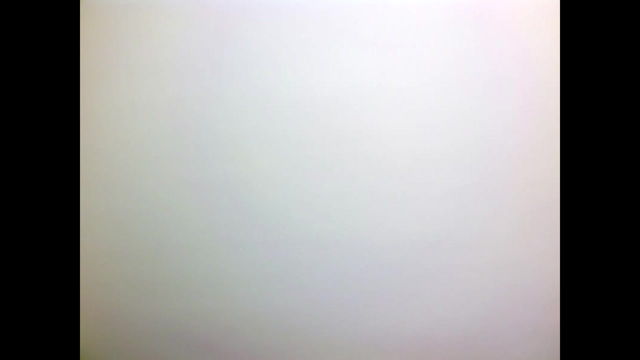 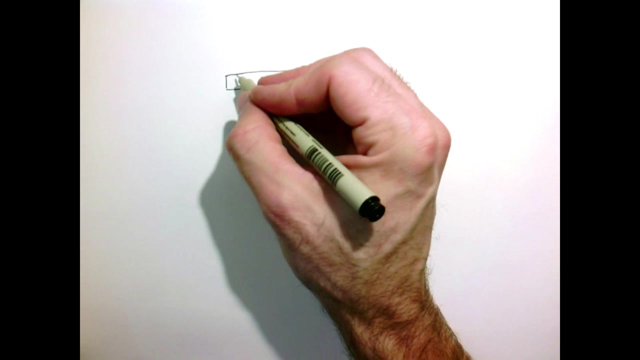 which could be a faulty assumption for high angles. Okay, now let's do a similar example as the last. Let's pay a little more closer attention to the viscous forces at this time. So let me just take my surface to be horizontal. 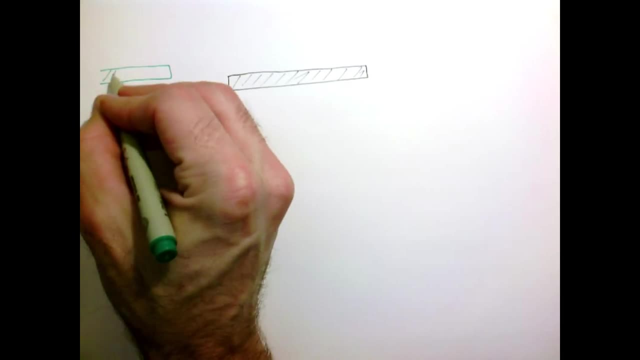 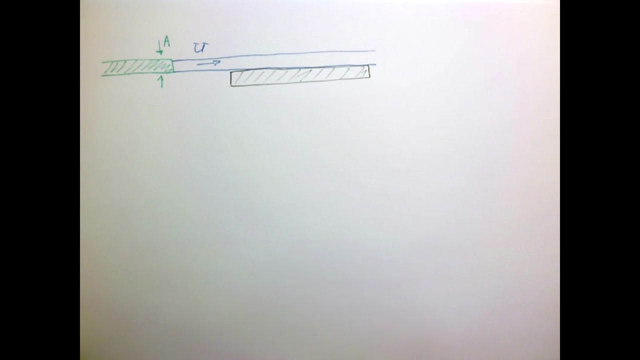 and again I'm going to spray a hose at this. Okay, so we're going to have kind of the same problem as last time, except I'm going to kind of relax one of my assumptions. So I'm still going to assume it's steady. so we're not interested in transients. 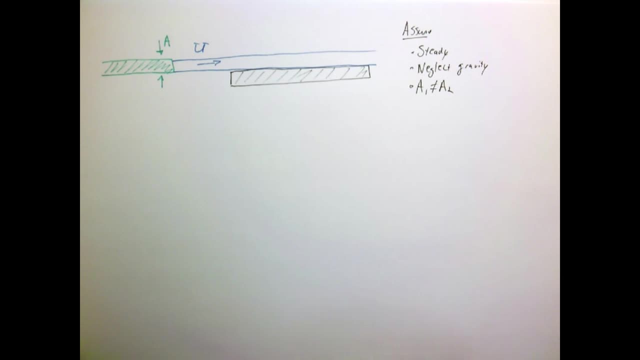 But now I'm going to relax the assumption that a1 is equal to a2, and by a1 and a2, I just mean we'll draw a control volume again to include the plate. I will call this surface 1,, this surface 2,. 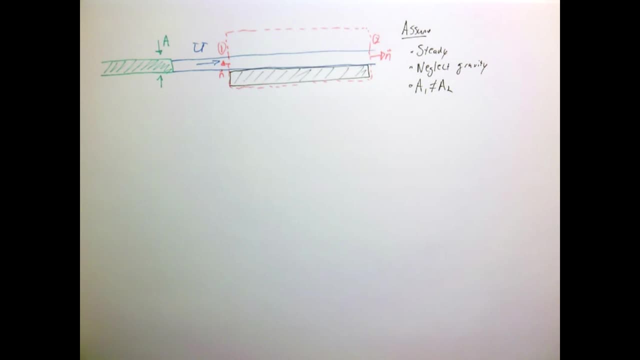 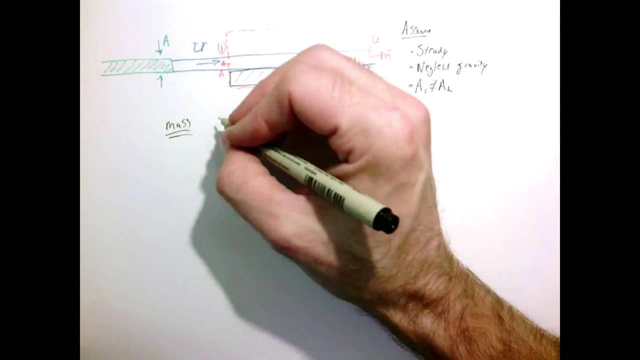 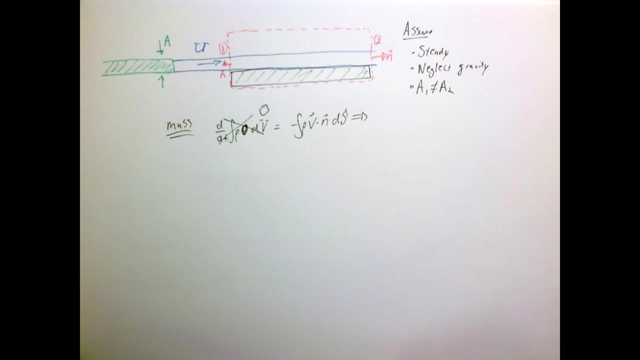 with normal vectors pointing outwards. So we're going to simply relax the assumption that a1 is equal to a2.. Conservation of mass: just like in the last problem, it's steady, so that term is going to go away. So we just have the flux of matter coming in and out. 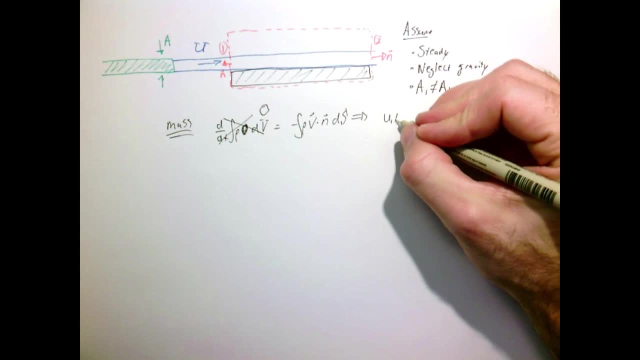 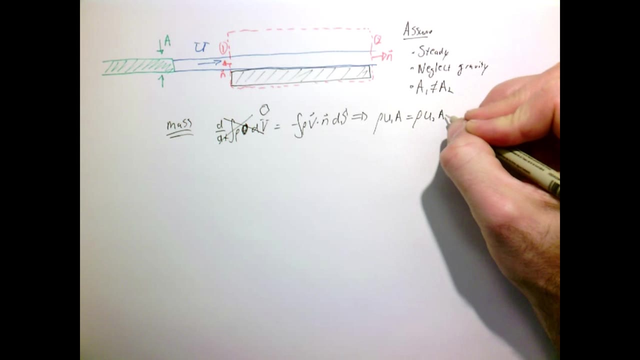 So here we have the velocity at 1 times the area at 1, times the density equals the velocity at 2, times the area at 2.. Now the density will cancel, but since we're going to relax the assumption that a1 is equal to a2,, 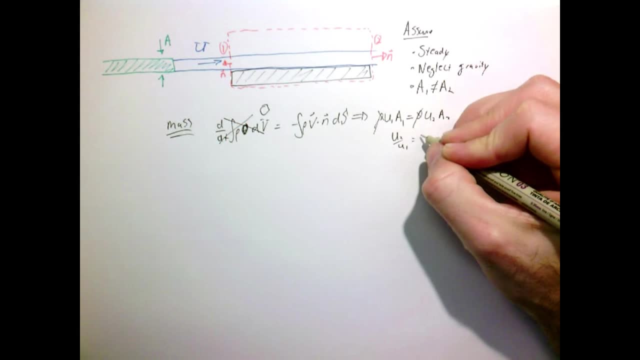 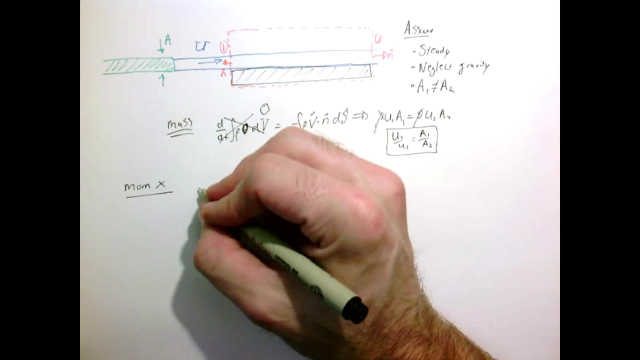 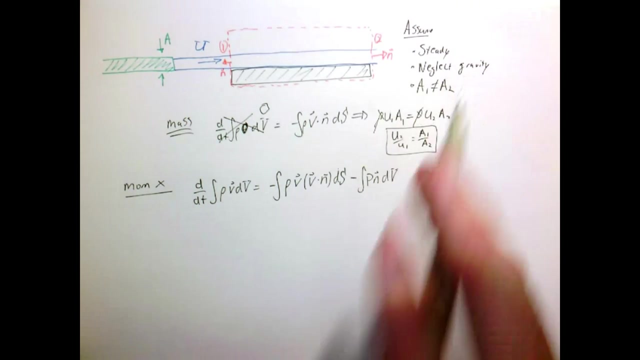 then we simply have that u2 over u1 is a1 over a2.. Now let's go to conservation of momentum. Here we only have x momentum to worry about. I'm not going to write the gravity term, because we're just going to cross it out in the end. 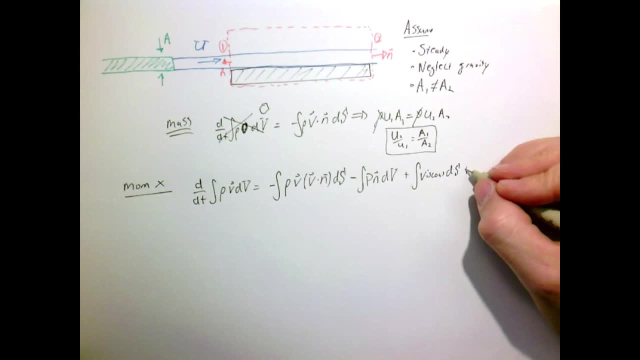 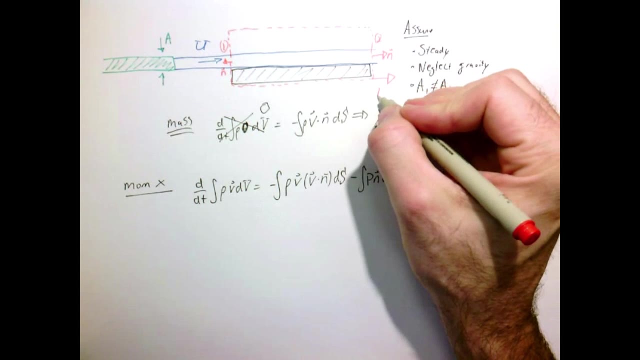 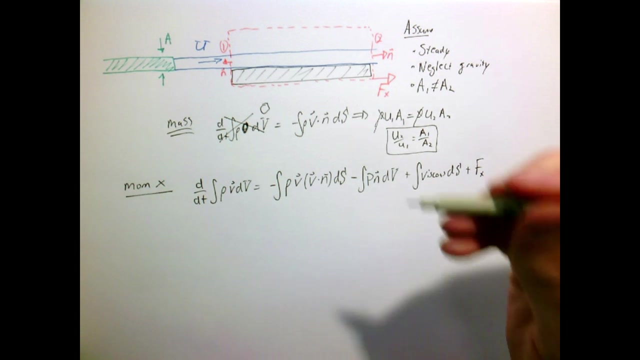 I have my viscous stresses that I'm just writing as the viscous plus my external force in the x direction, because again I need to apply some force to this plate to hold it in place, presumably So, as before, we have p atmosphere. 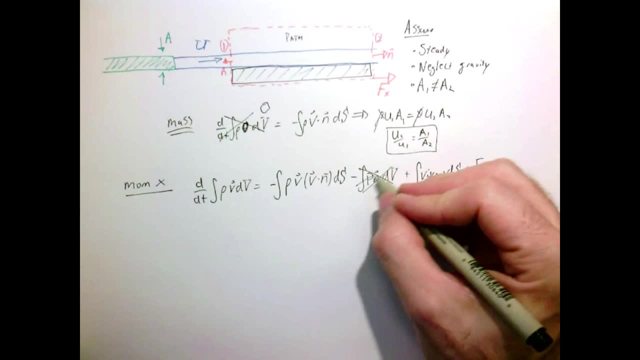 It's a jet that's free in air and so, by the same argument as before, we're really not going to have any pressure to worry about. The pressure is just, and the whole system is basically going to be at p atmosphere, so the pressure term isn't going to do much. 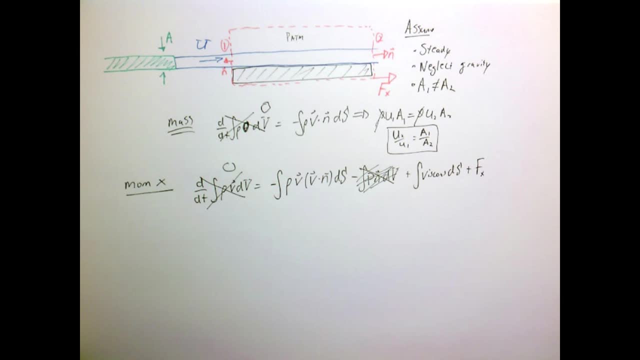 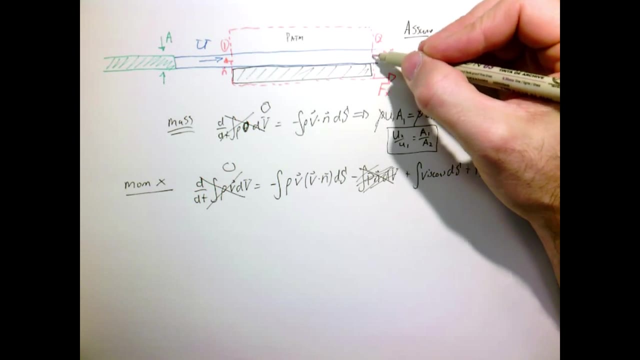 It's steady, so that can be 0.. And again by the same argument as before, the viscous stresses here, at this exit, here where the jet is free, and at the entrance, where the jet is free, are basically going to be approximately 0.. 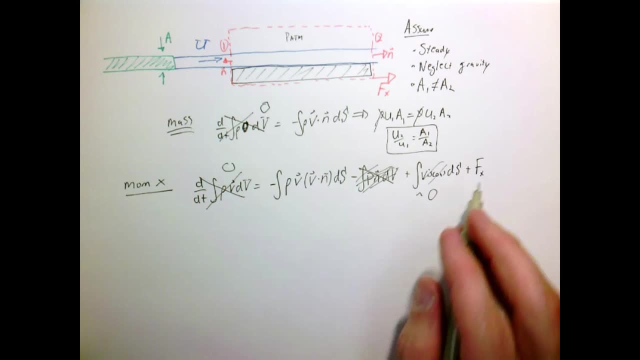 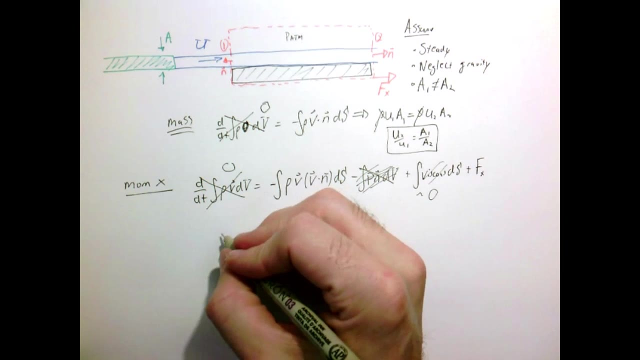 So I'm going to neglect those. So we have the same expression as before, where the external force is the change in the flux of the momentum. so let's work out what that is And, again, let's be careful about our sign. So we have a negative that comes from here. 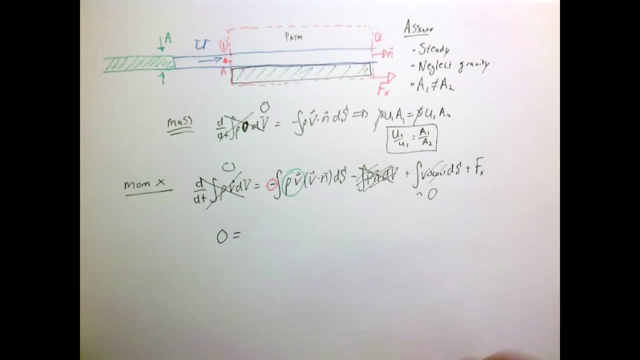 a sign that shows up in the velocity vector and a sign that shows up in v dot n. So again, I've been careful of my sign. I get a negative sign here and I've got a negative sign in this term because v dot n is negative, because the velocity and the normal vector are not aligned at state 1.. 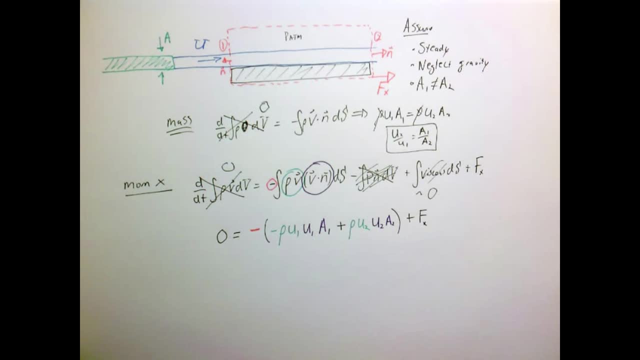 Here it's positive and that's my force in the x direction. Now we might notice from conservation of mass: u1 a1 equals u2 a2.. So this u2 a2, I can cross out and substitute with u1 a1,. 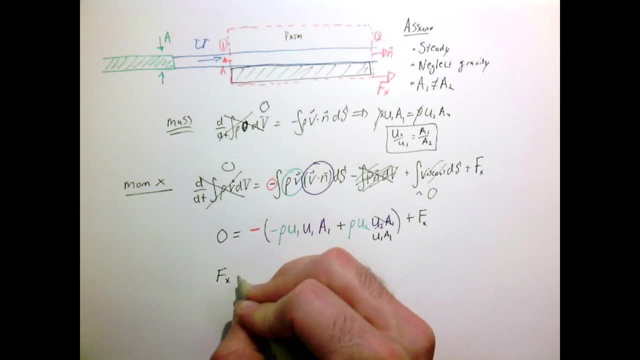 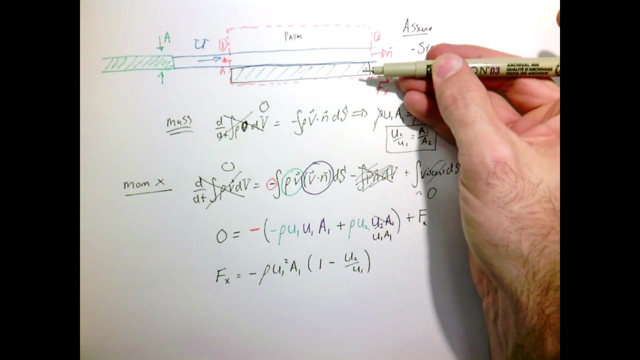 and I could rearrange this expression to be: the force in x is minus that. So we expect the force to be negative because I expect that I'd have to hold the plate in place, otherwise it tends to want to move in that direction. 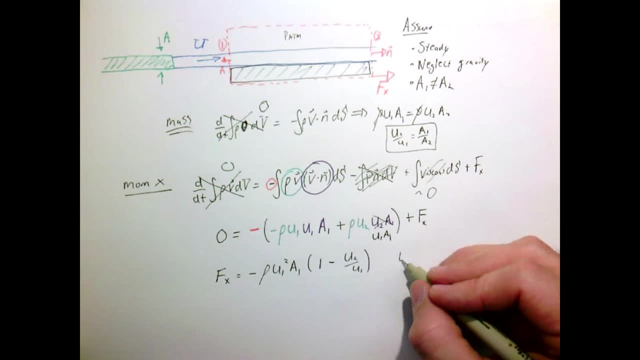 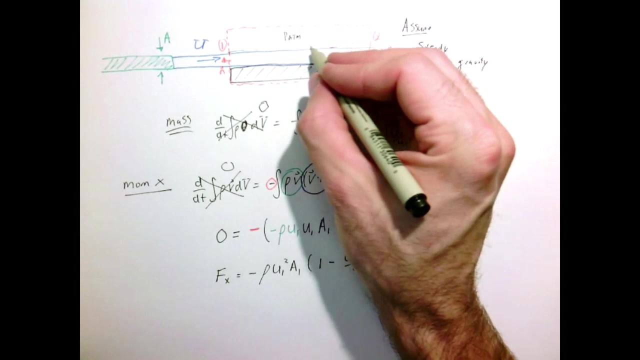 And so that tells us that u2 should be less than u1, which, if we look at this expression here, tells us that a2 should be greater than a1. So the jet should come in narrow and fast and it should thicken a little bit if it does anything. 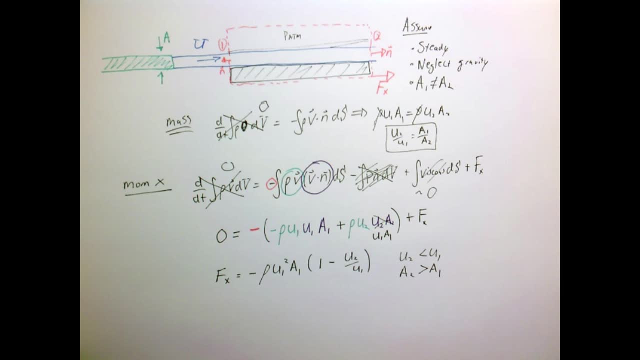 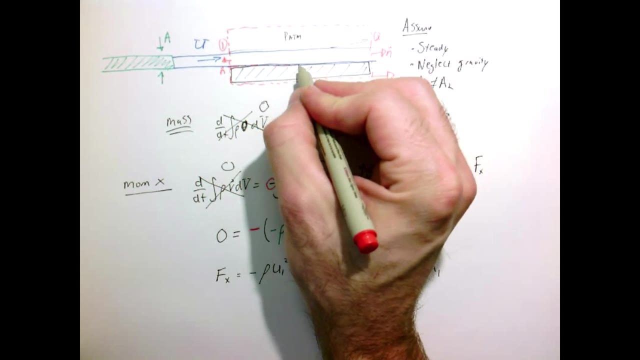 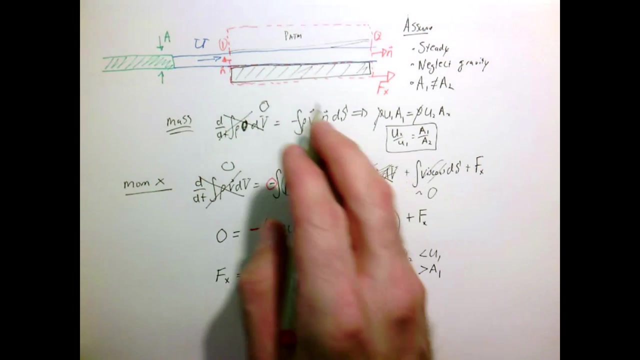 Now we can relate how much it's thickening or what's going on here to the viscous stresses. because if you imagine, instead of the control volume I drew I cut right along this surface here, then just Newton's law is what tells us the force has to be equal and opposite at the surface. if I slice it here, 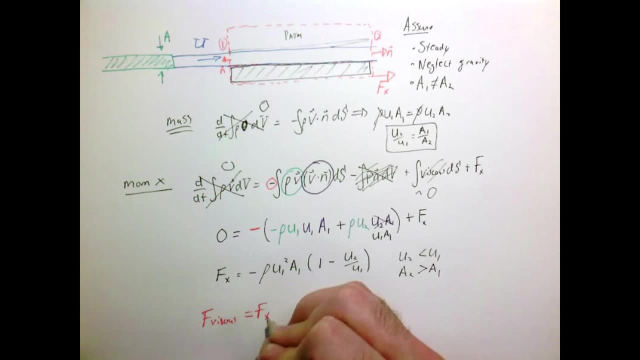 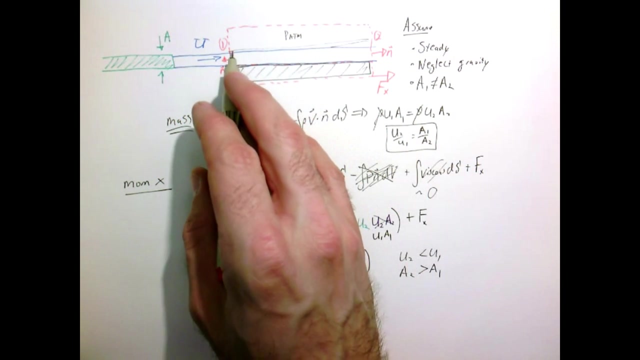 tells me that the viscous stresses have to equal this force that we're holding things in with, And so what that means is that this term here, if there are any viscous stresses acting on this surface along here, if we have viscous stresses along here, our momentum balance would tell us that we expect this. 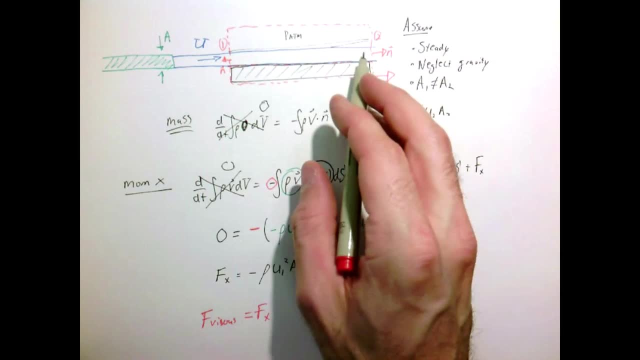 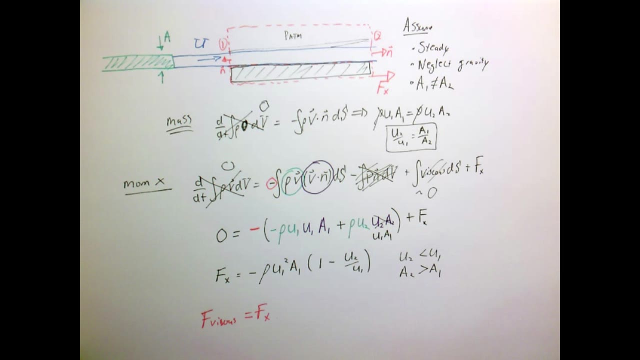 jet to thicken and become slower, so it has more momentum coming in than out, which is sort of offsetting the forces which are going in that direction. And so if there are viscous stresses that we want to worry about our conservation momentum doesn't give us any way to 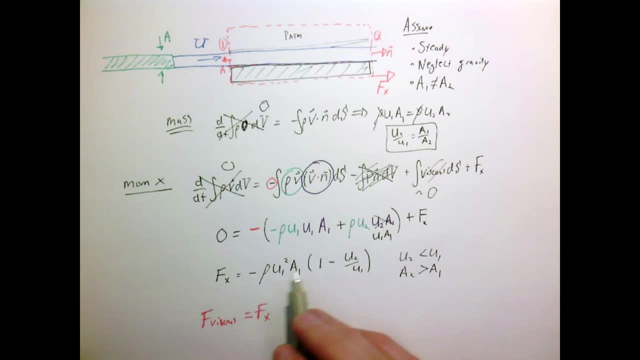 actually calculate what those are unless we make some other assumptions. but it does tell us the direction things go and the fact that if in fact there are viscous stresses, this thing needs to thicken and A1 is not equal to A2.. So in the previous problem, 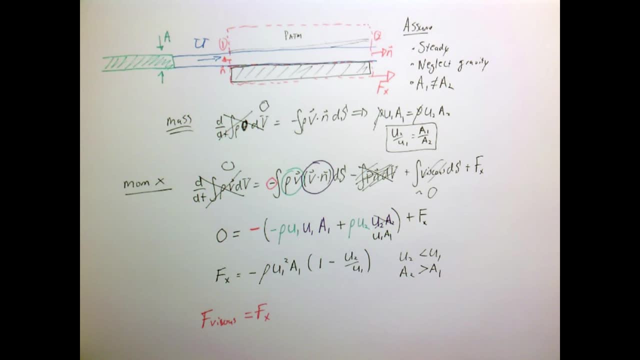 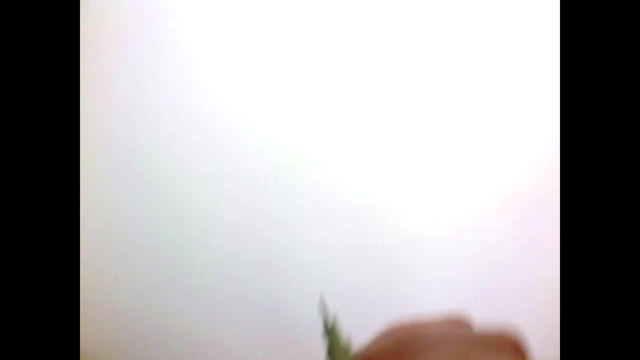 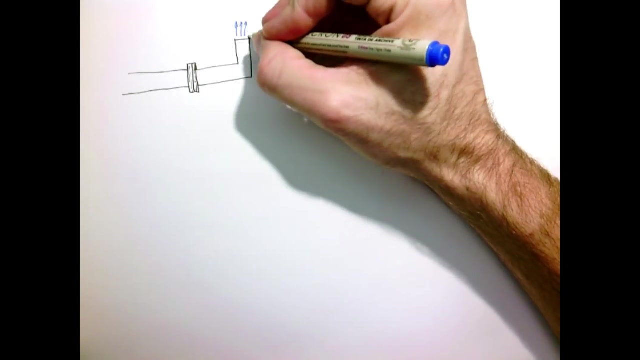 where we assume that A1 equal to A2, that would be consistent with assuming that the viscous stresses are negligible along the surface. Okay, let's just move on with a few more examples, just to sort of see how things work. Okay, so let's assume we have a 90-degree bend. 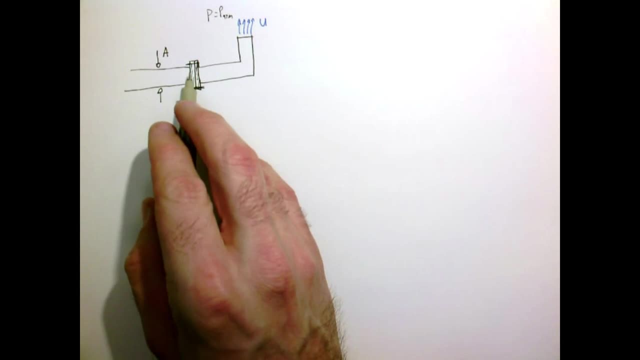 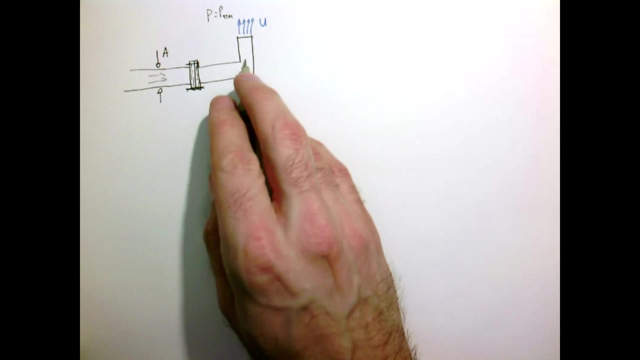 We have a flange here which is bolted together to a pipe so we have fluid flowing in our pipe here. The exit velocity here is U. The pipe is size cross-sectional area A everywhere along here, so we won't worry about the area change. but there's sort of this 90-degree bend right at the exit. 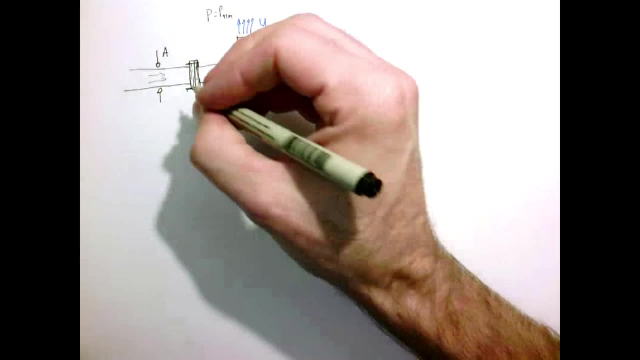 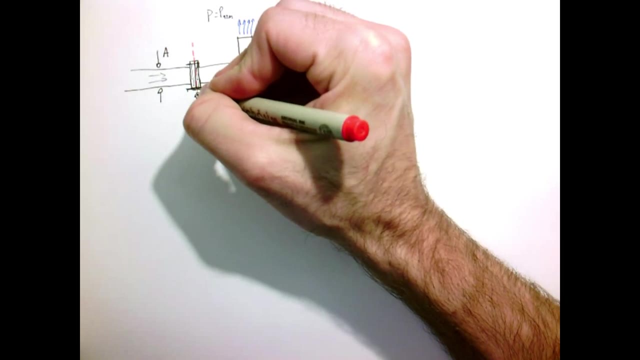 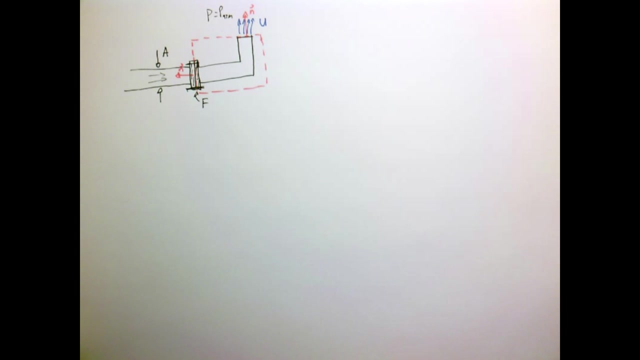 And what we want to know is: what are the forces that are acting on these bolts here? So what force do we need to hold this thing in place? So we'll draw a control volume to cut. like that We have normal vectors pointing out in that direction. 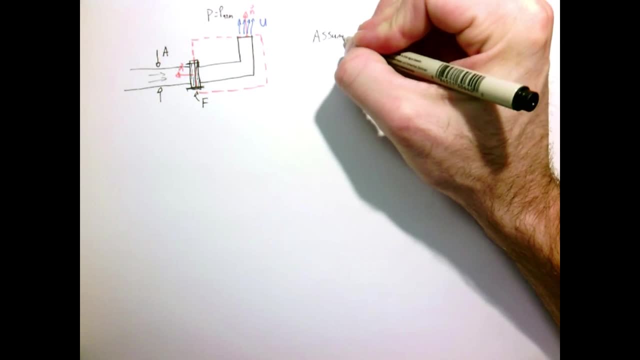 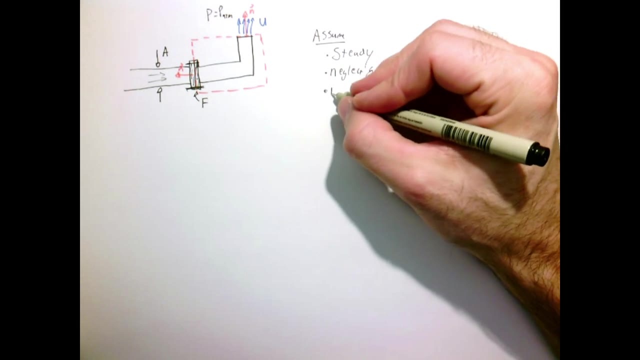 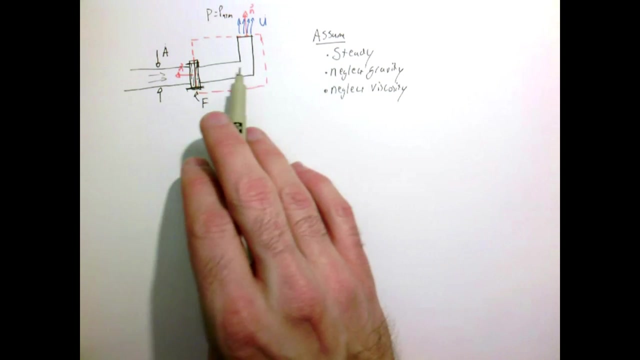 And now we need to talk about what our assumptions are. Ignore transients at steady. Let's neglect gravity. We're gonna neglect viscosity. so we'll assume there's no viscous stresses. So we're just interested in how much momentum there is, but by turning it wants to sort of pop this little 90-degree bend off. 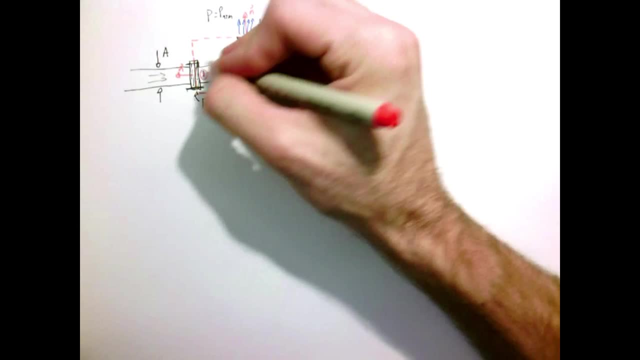 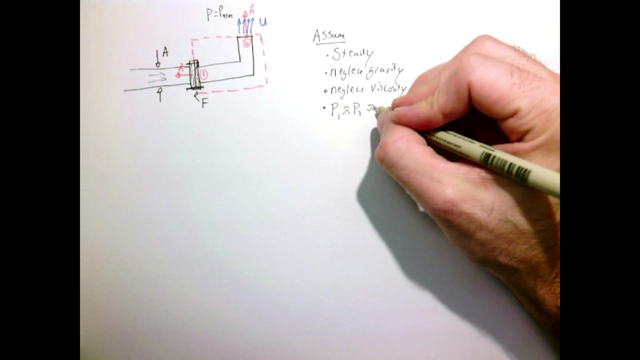 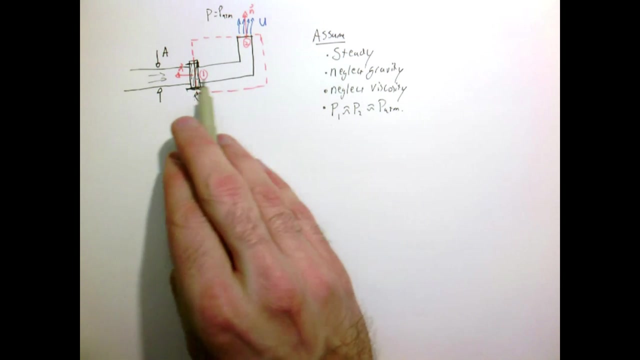 And finally, let's assume, if we label these surfaces 1 and 2, let's assume, that the pressure at 1 is approximately the pressure at 2, is approximately the pressure of the atmosphere. So there's basically no real pressure loss around this last little bit of the bend. so the pressure doesn't change much between here and here. Now, in reality, 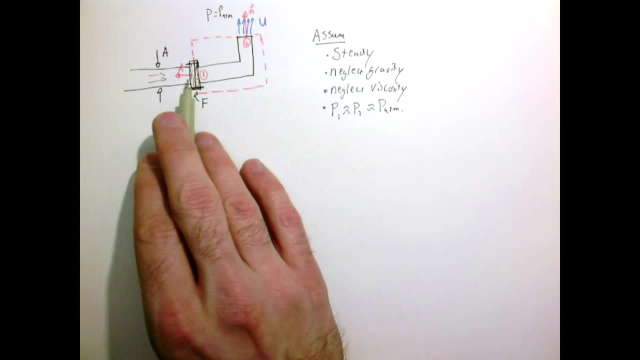 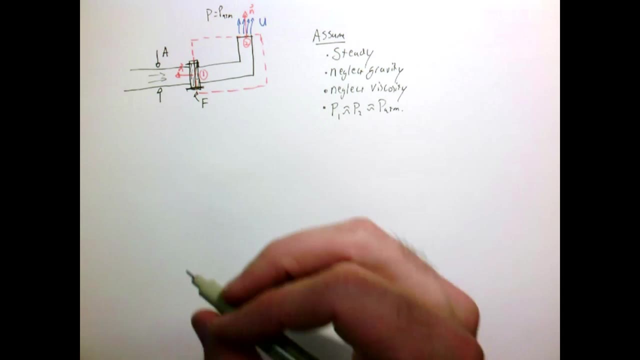 this pressure would be a little bit higher, which would exert a force. maybe that would be a little extra than we'll calculate for wanting to pop this thing off, but we'll just assume that there's basically no losses in this bend. So let's write out our conservation of momentum. 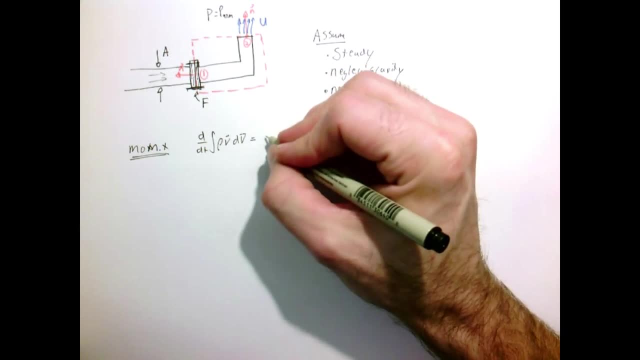 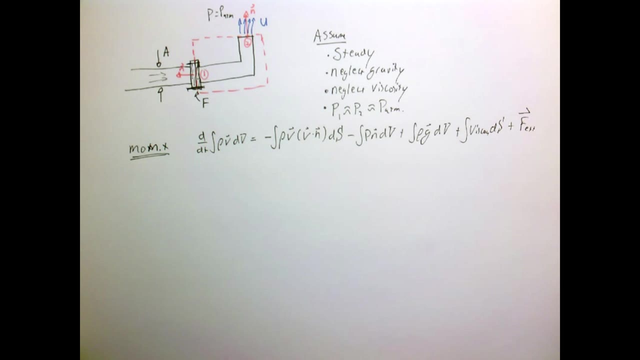 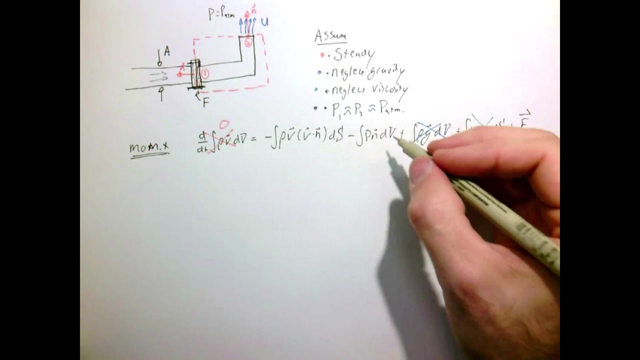 in the x direction. So there's all our terms. By the steady assumption that one goes away By neglecting gravity, that one goes away By neglecting viscosity, that one goes away And by saying the pressure is basically everywhere, p-atmosphere, that term goes away. 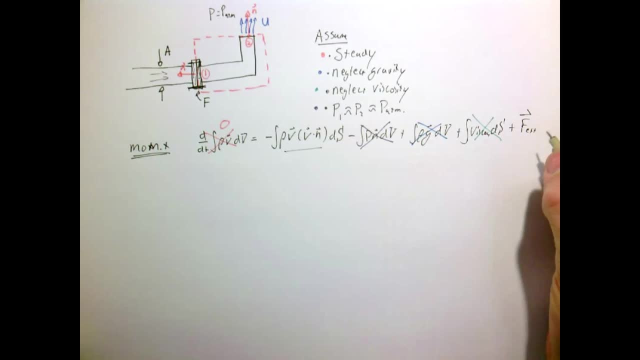 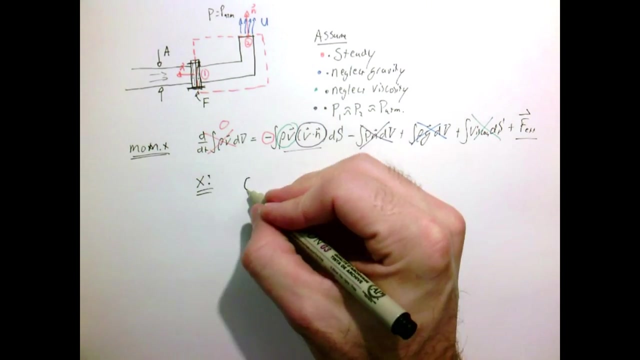 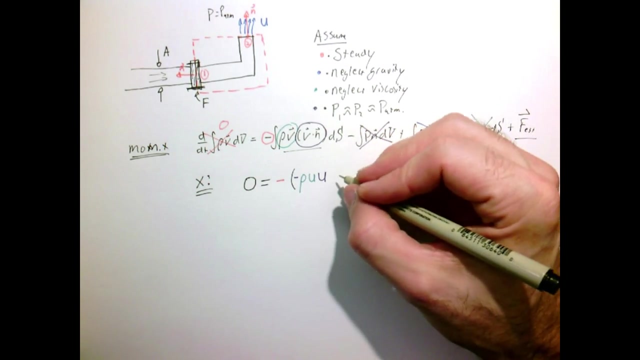 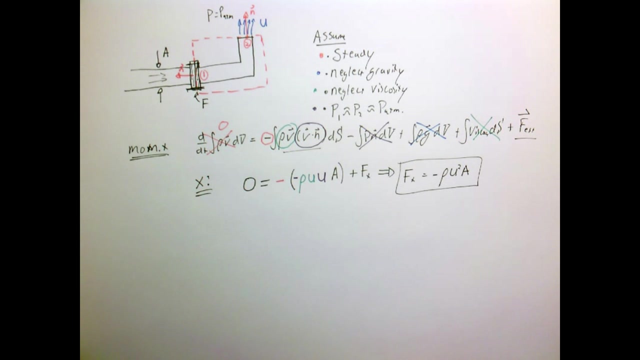 So all we're left with then is the flux of momentum and the external force. So when we do the x-component of the momentum, let's again be careful with our signs. So for the x-momentum, there's velocity here, right? So rho v is just rho u on this one, which is that term there. 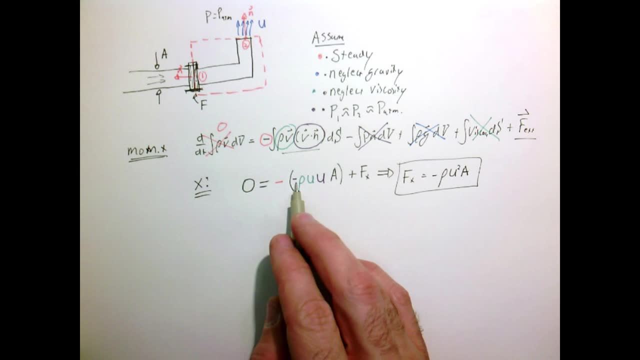 And v dot n is u, but with a negative sign. so that's that term. But at this surface, at 2, there's no x-component of the momentum, so it's just zero. So we only have x-momentum here which is being turned, and that has to be balanced by f of x. 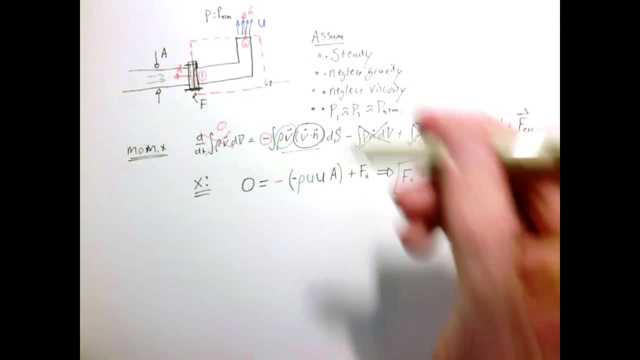 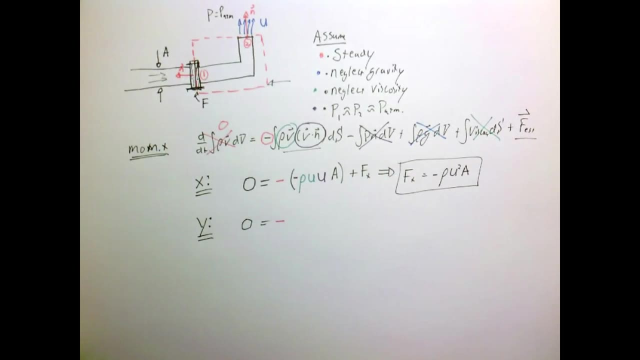 which is pushing back on this thing, because it turns out to be negative. So it's our force holding that in Our y-momentum will be very similar. so we'll have zero Because rho v is just rho u, because the velocity here is the same as the velocity here. 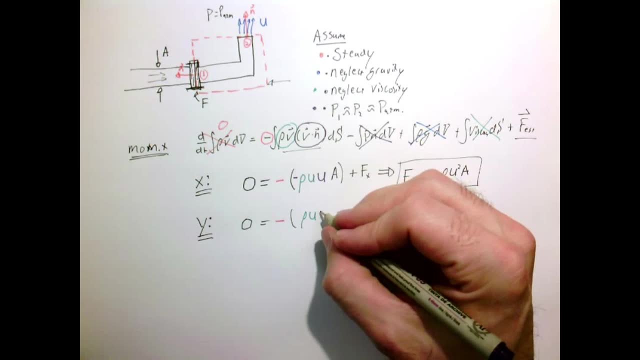 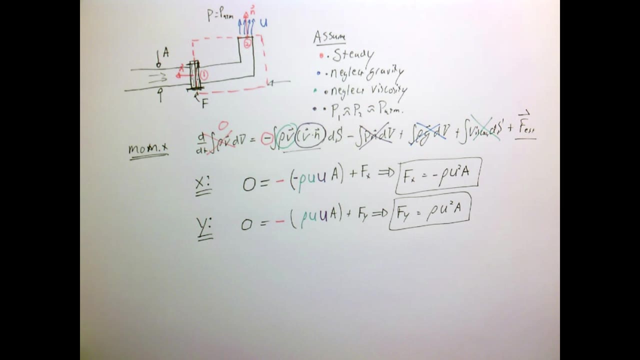 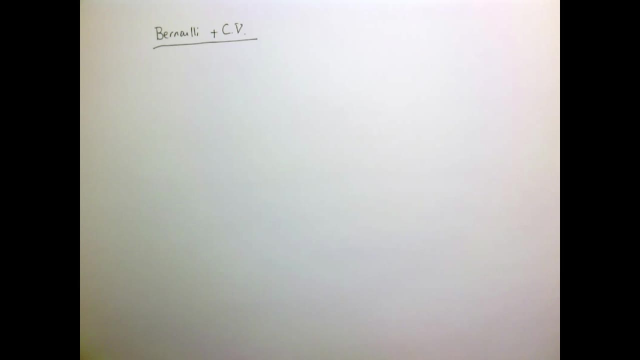 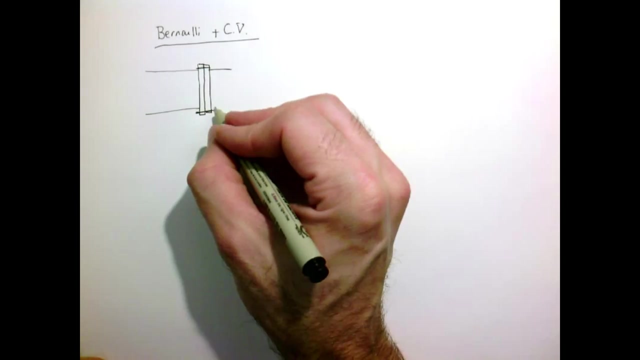 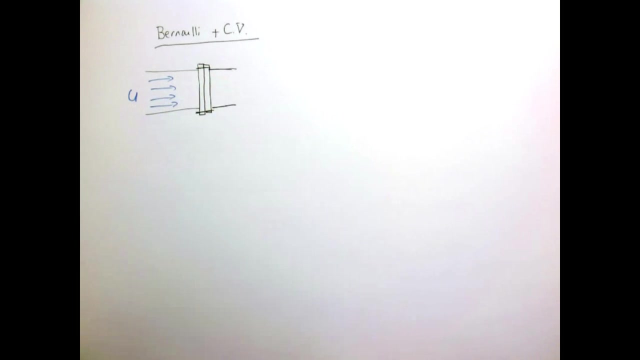 Now let's do one where we apply Bernoulli's equation and a control volume. So again we're going to have a pipe with a flange where we want to know essentially the force on those bolts that's holding this pipe together. We have velocity U here, except now we're going to have a nozzle that comes down, reduces. 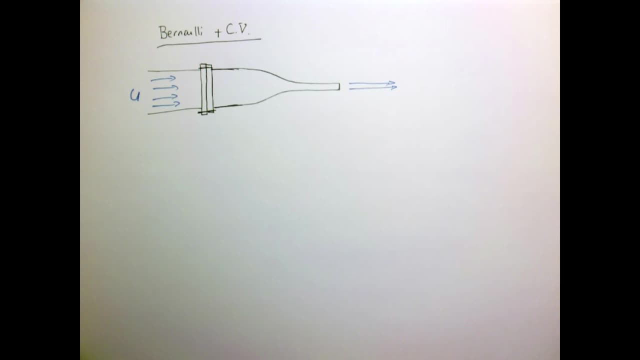 in diameter, so it squirts out a lot faster than it comes in. Upstream we're going to have area A1, downstream we're going to have area A2.. Upstream we're going to have velocity U1, downstream we're going to have velocity U2.. 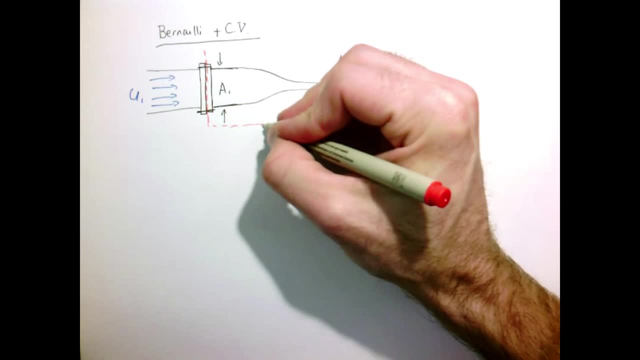 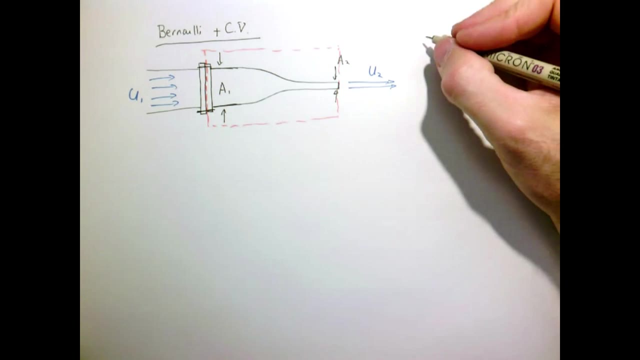 Now in this problem, we'll draw a control volume to go right down, cut directly, like that Seems like the obvious choice. And now we're going to talk about what our assumptions are, Again, steady, So we're going to assume the flow is steady. 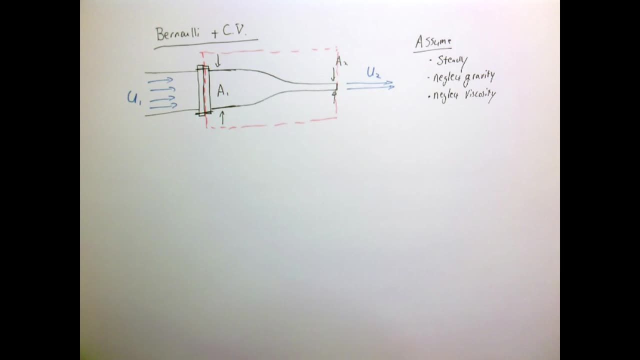 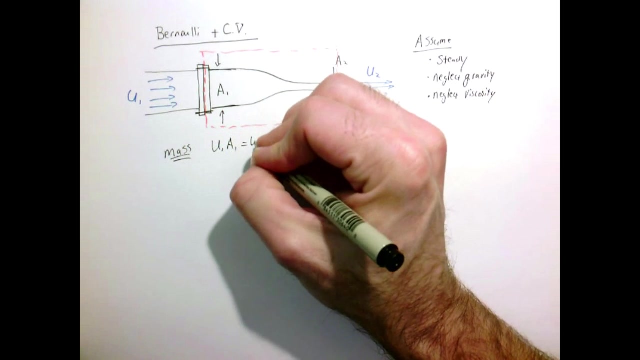 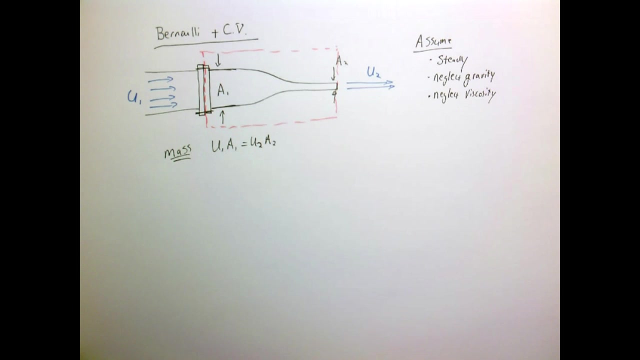 We're going to Neglect gravity, we're going to neglect viscosity. Now we could write it out, but I think we know by now that conservation of mass is going to give us the following relationship: It's going to tell us that U1 times A1 equals U2 times A2.. 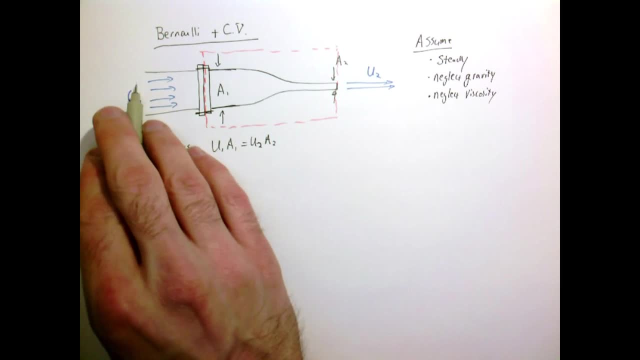 Now we should note when we write this, what we're really assuming is the velocity profile here is roughly uniform or we can capture it as such, So a mean velocity times the area is kind of good enough For our analysis. So we're not really worried about the velocity profile here, whether it's a parabola or some. 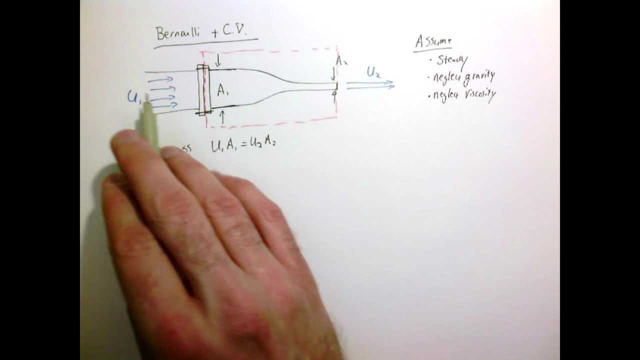 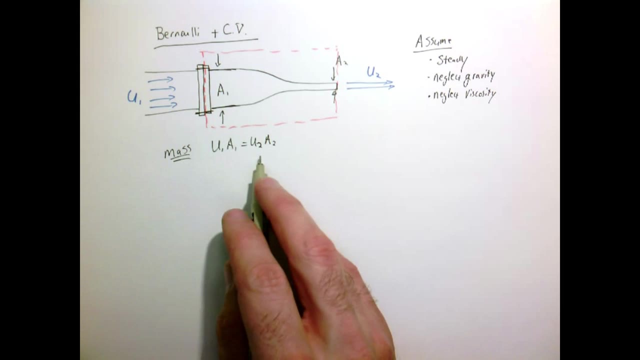 other shape. But since we're neglecting viscosity and it's high speed, it's usually a pretty good assumption to assume that things are rather blunt and at least in a net sense uniform. So that is an assumption that we're really not solving for the detailed velocity profile. 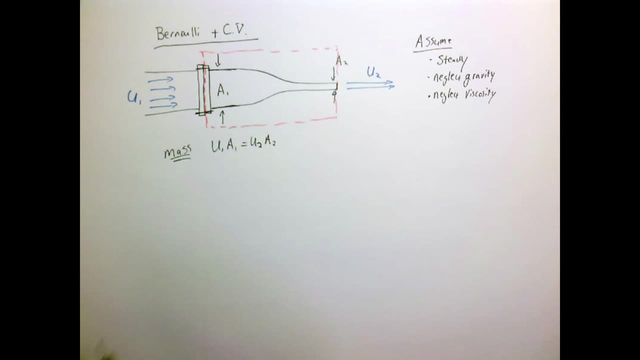 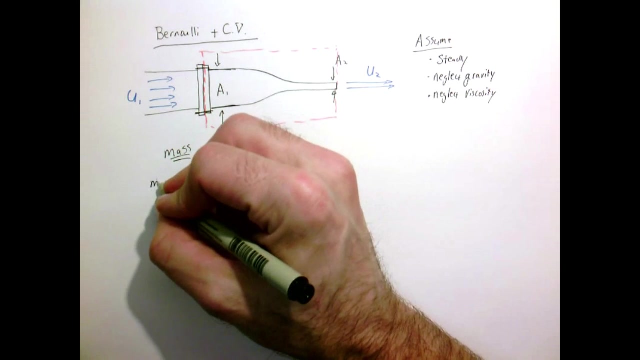 We're just saying it's basically uniform, So it's just the velocity times, the area to get the total flux of mass crossing the surface. Okay, Now let's do momentum and we'll write all our terms out. Okay, And here we're really only going to have momentum in the X direction because there's 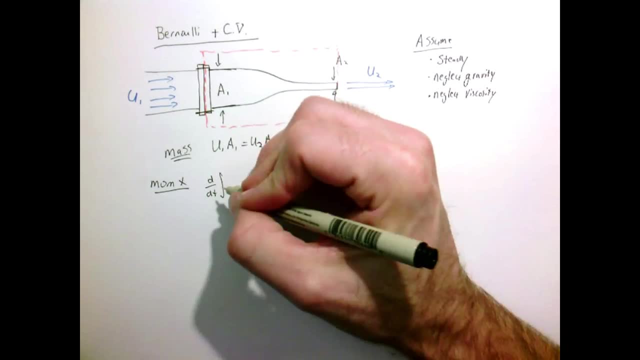 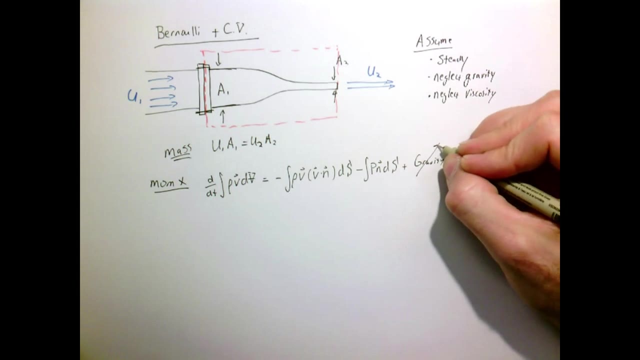 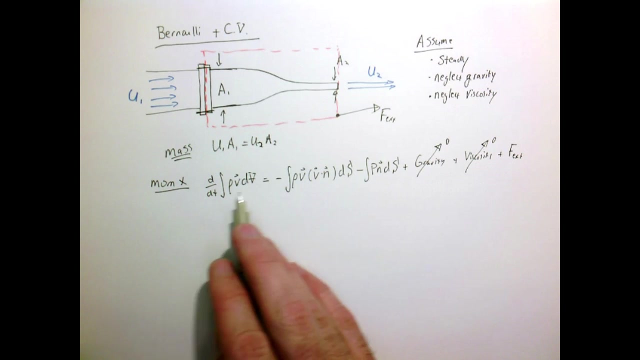 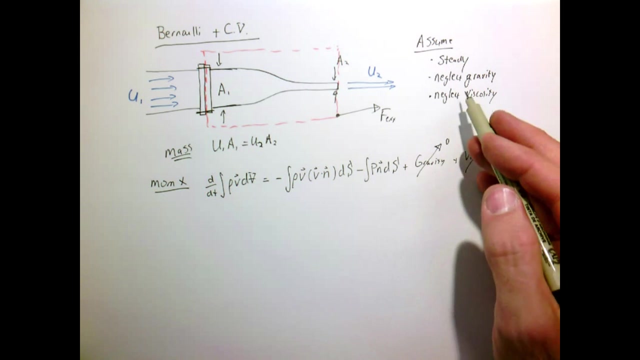 nothing happening in the vertical direction. So again we have the change of momentum in the control volume. so it's the net flux in and out, the net force due to pressure, gravity, viscosity, and our external force by our assumptions of neglecting gravity and viscosity. 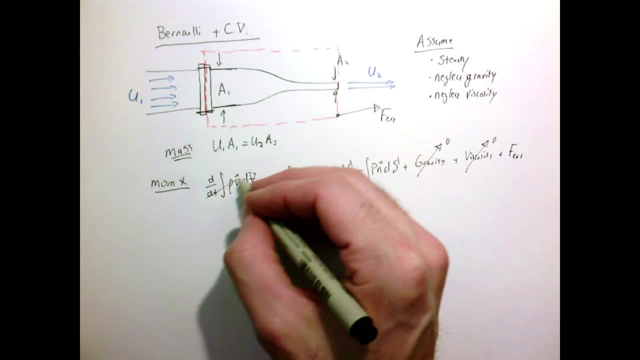 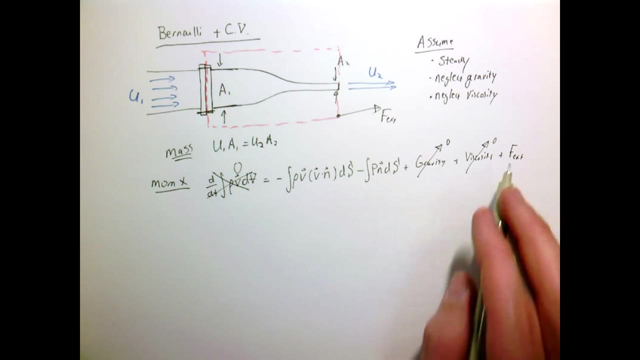 I'm not even going to write those out, They're just zero, And by our assumption of steady I could also just say that that's equal to zero. So now we have net flux of momentum in and out of our box pressure and our external. 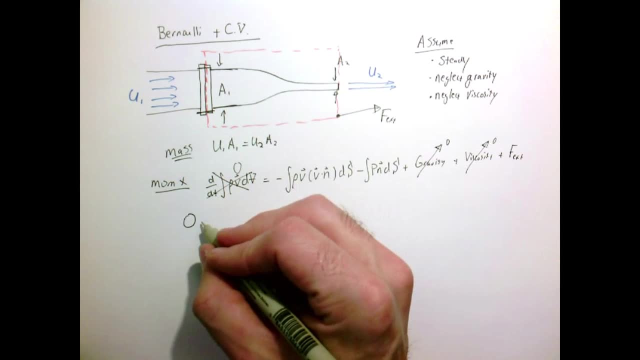 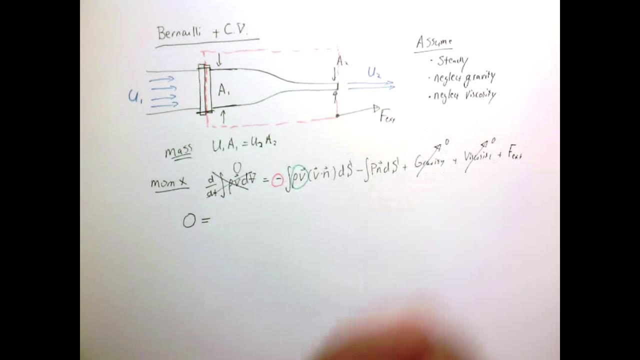 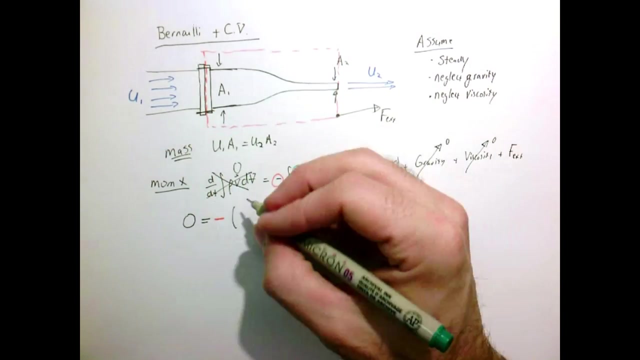 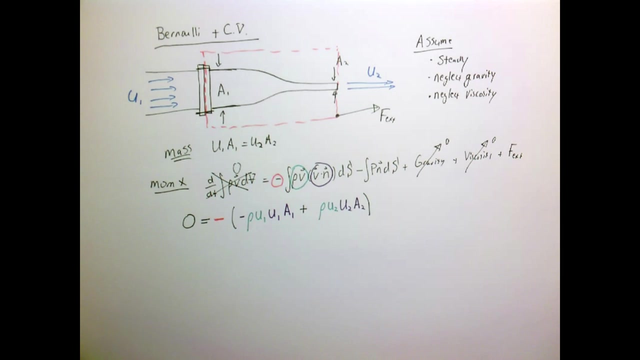 force. So again, being careful with signs to make sure we get everything correct, We have this negative sign to worry about, the sign here of rho V and our sign here with V dot n. Okay, So, as before, we have the sign of rho U, which is going to be U1 and U2, at entrance. 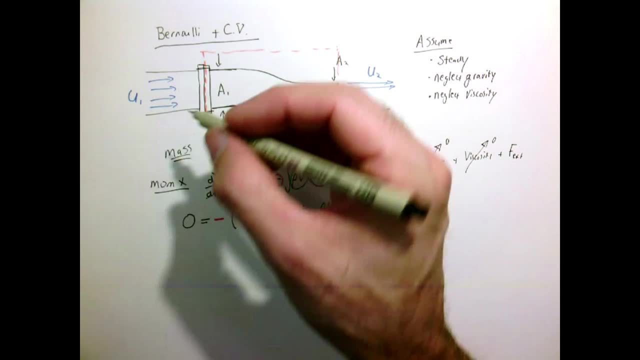 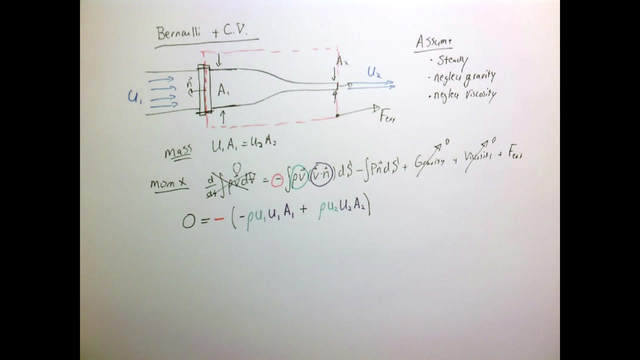 and exit. We're going to have U dot n being negative here because our normal vector points out. We're going to have U dot n being positive on this side because the normal vector points out. So we've seen all this before. Now let's do the pressure. 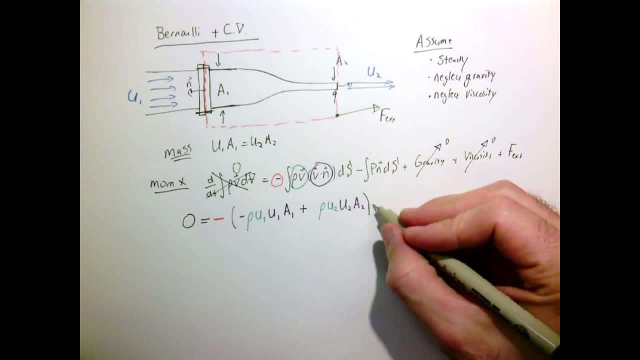 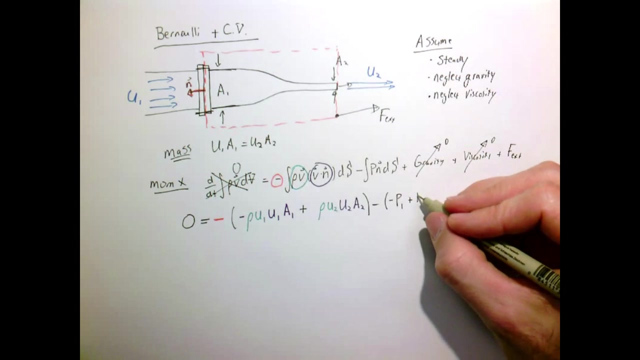 The pressure we have to be a little bit more careful about. So we have a negative sign here And at surface one the normal vector points outward in a negative direction. So we have minus P at one, We have plus the pressure at two. 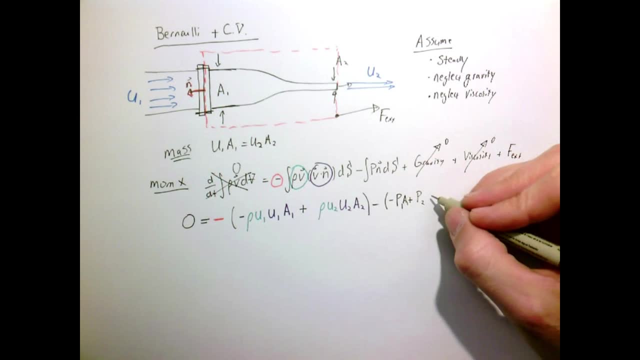 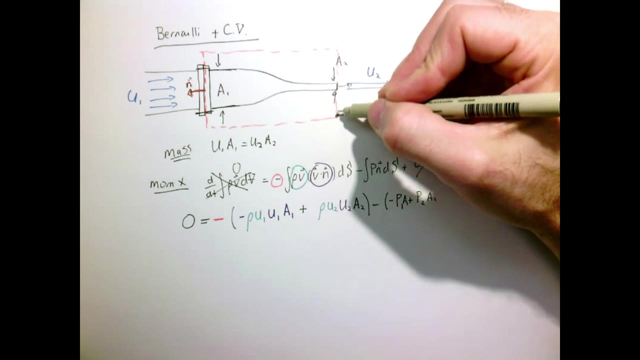 Now I need to be careful at the area. So this is going to be A1.. This is going to be A2.. But we have to be careful of the rest of the control volume as well, because we have to consider the pressure acting on every surface. 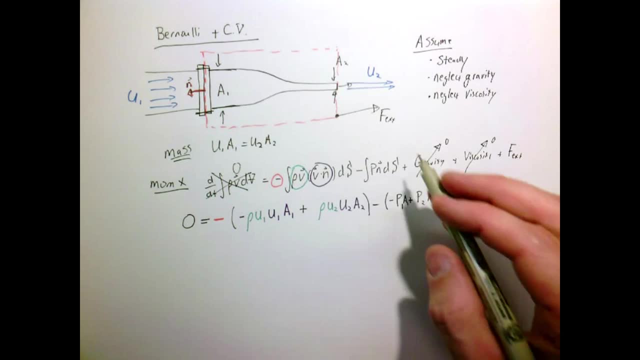 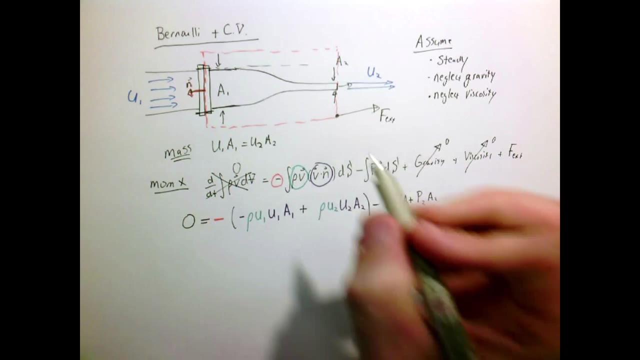 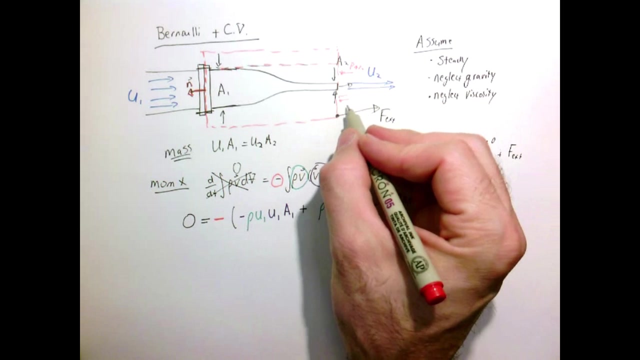 So here We have the pressure of the fluid at the exit times: A2. But we have over this- I should draw that in red- actually over this projected area, we also have the pressure of the atmosphere And it's pushing back in the negative direction. 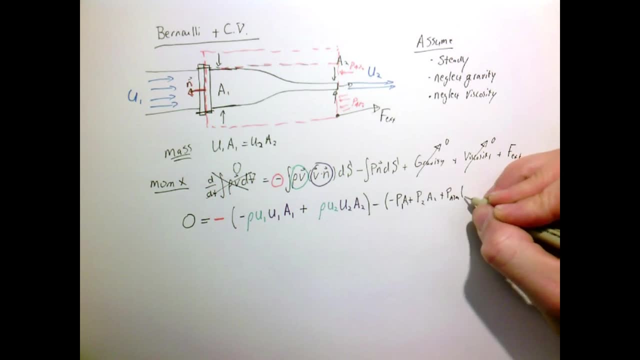 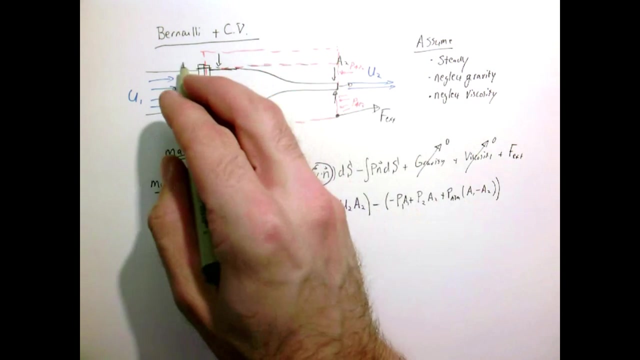 So I'm going to add it as plus P atmosphere times A1 minus A2.. Acting over that stuff Now, we could also worry about the pressure acting here, But once we're outside the pipe, atmospheric pressure pushes this way and pushes that way. 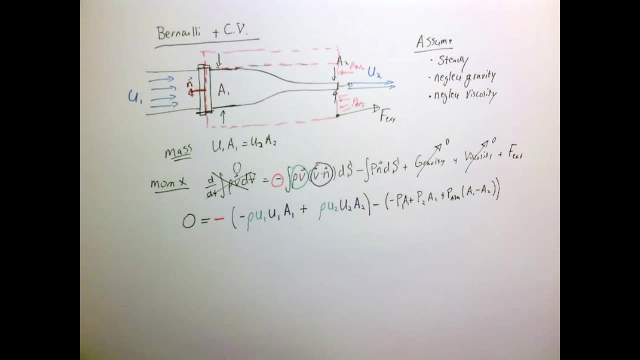 so it balances. So I'm just going to worry about the area just around the pipe, And that has to equal our external force. Now, however, since this jet is exiting to the air, and it's just exiting in straight lines, the pressure of the atmosphere is the pressure of the jet. 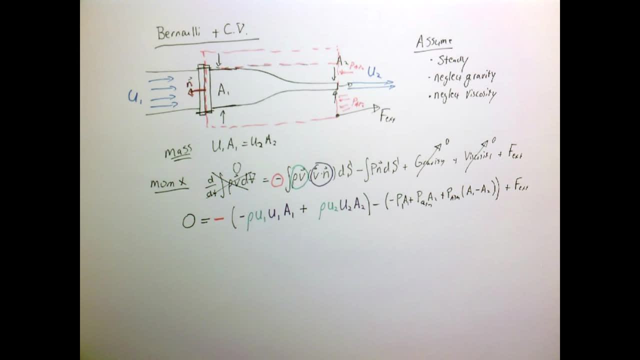 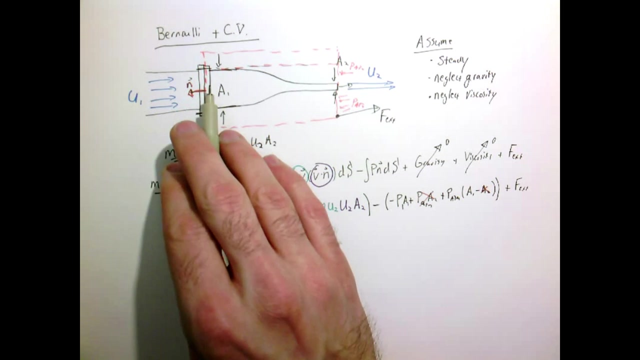 So we can substitute The pressure at 2 with P atmosphere, And now we see that P atmosphere times A2, P atmosphere minus A2. This term will cancel with that term, And so the net force due to pressure is just the pressure at 1 relative to the atmosphere. 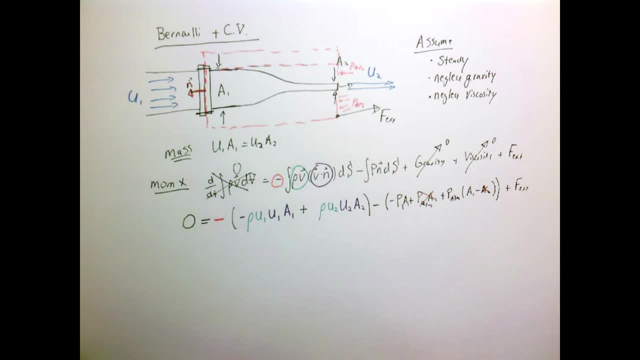 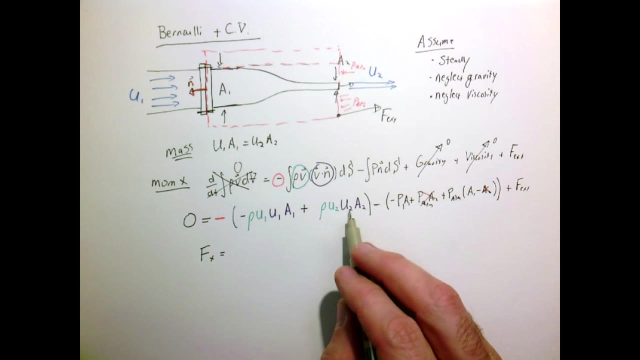 times the area of 1.. So let's write all our terms out and see what we think about the sine. So our F of X. Let me make one last change. So we have U2A2,, U2A2, that's the same thing as U1A1.. 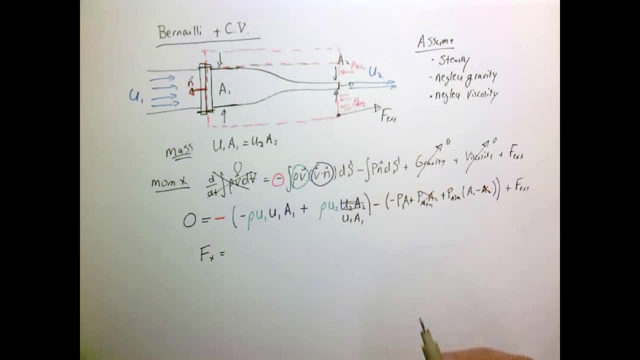 So I can cross those out. This is U1A1.. So when I rearrange the terms to one side, we have the force is equal to some change in momentum term which we'll have to work on just a little bit more times. pressure. 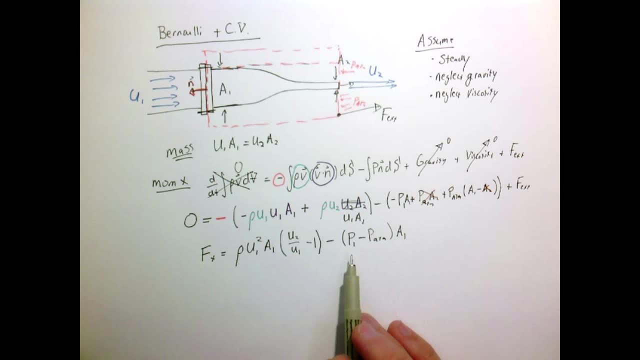 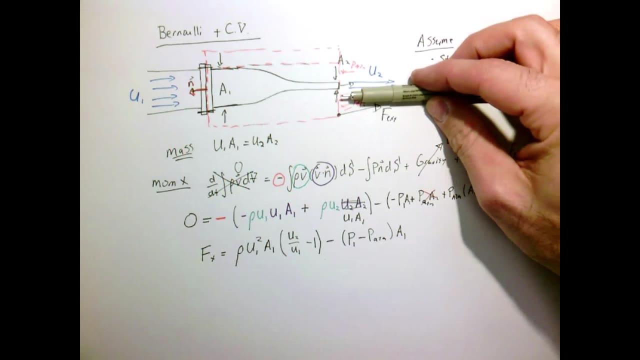 at 1 minus the pressure of the atmosphere. So let's think about the sine of this term, This term here: if this pressure is higher than atmospheric, this is positive. So it wants to pop the nozzle off. so we have to exert a force in that direction. 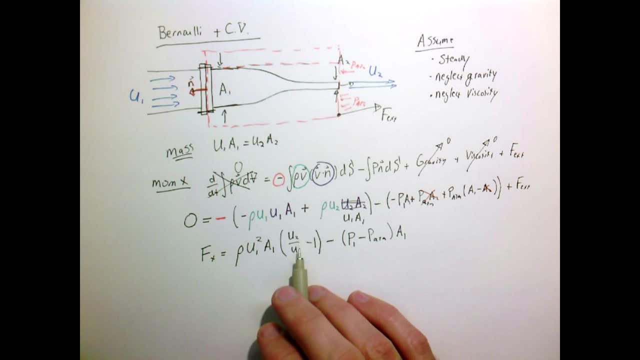 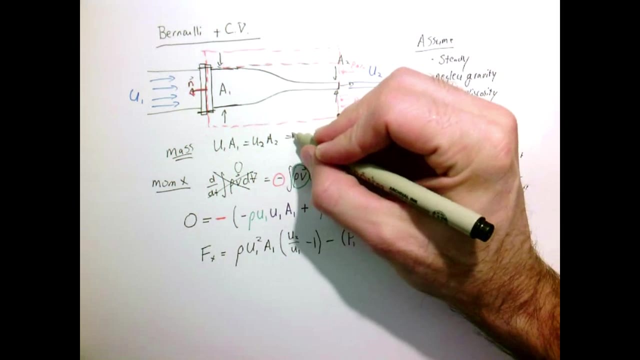 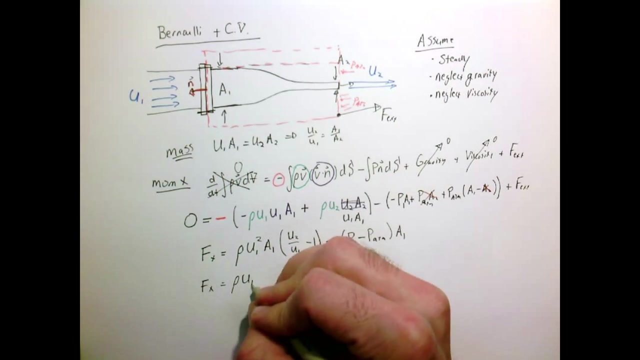 So I like the sine of these terms: U2 over U1. here we can also replace with A2 over A1, right, Because our conservation of mass would tell us that U2 over U1 equals A1 over A2.. So there's our expression for now for the force. 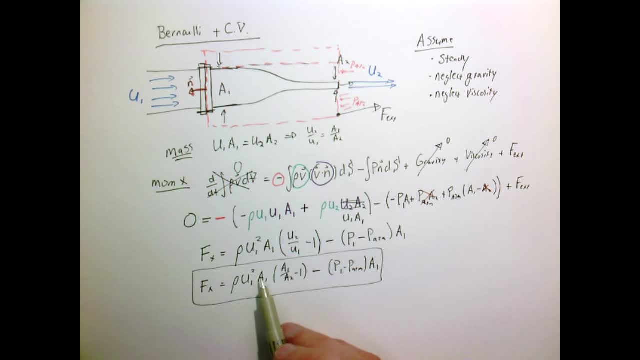 If we look at it, A1 is greater than A2, so this term is positive. We expect P1 to be greater than P- atmosphere perhaps, which would tend to pop that off. So it's not clear what the sine of this thing is, because we sort of have pressure and velocity. 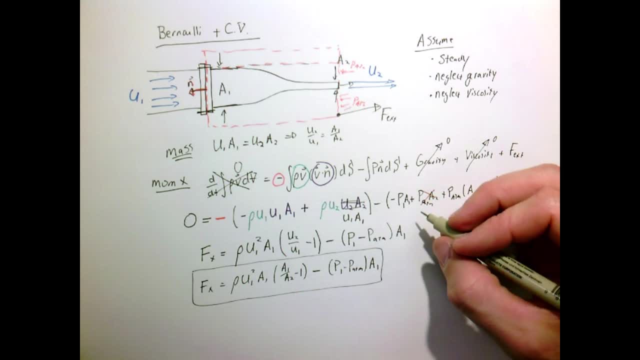 So we can make a little bit of progress here if we actually apply Bernoulli's equation. So let's apply Bernoulli's equation along the streamline running from 1 to 2, right down the middle. So we'll do that over here. 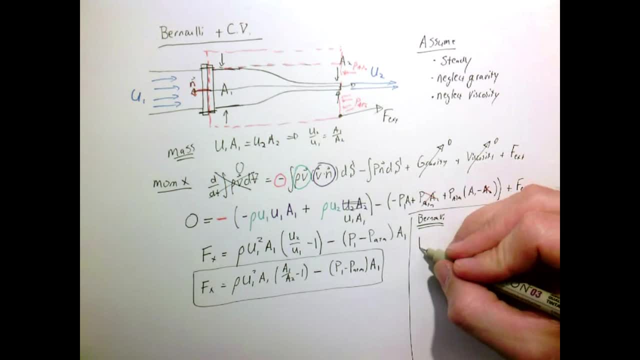 So that's going to tell us that the pressure at 1 plus 1 half rho U1 squared equals the pressure at 2, which is P atmosphere plus 1 half rho U2 squared. So I can rearrange this to be P1 minus P atmosphere equals 1 half rho U1 squared minus. 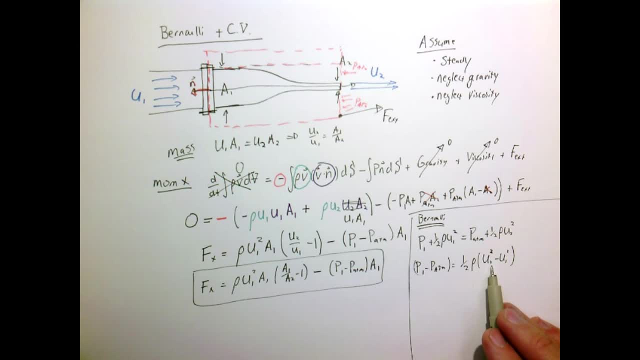 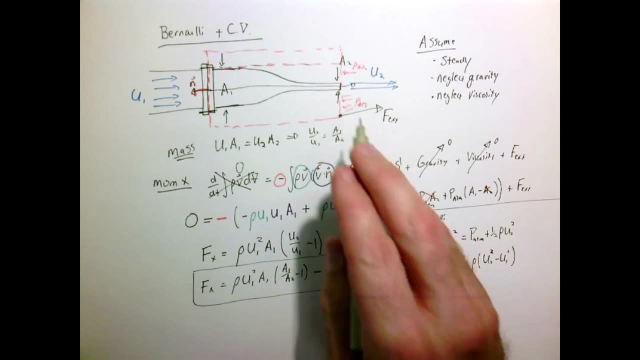 U2 squared, which is going to be a positive number because U2 is going to be greater than U1. So this is going to be a positive number. So we expect the pressure at 1 to be greater than the pressure here at the exit, which. 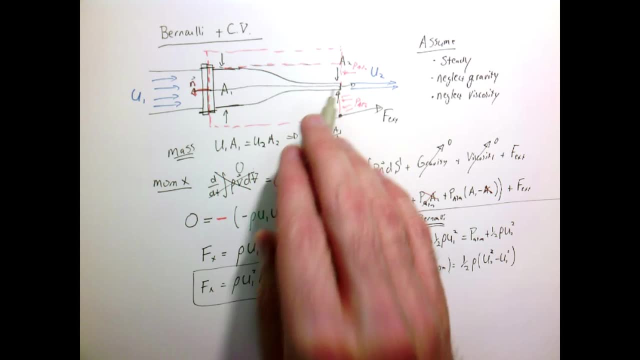 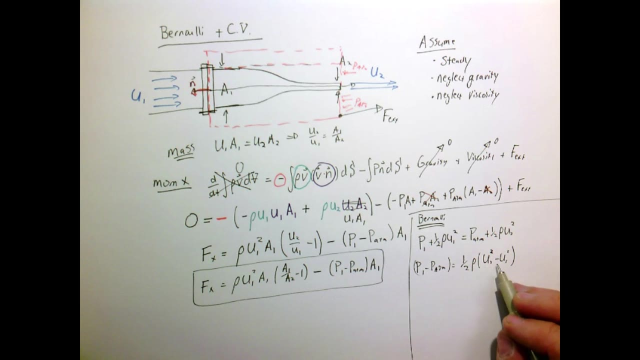 makes sense from Bernoulli's equation, because the velocity is high here, so the pressure is low. So we can substitute this expression into here for P1 minus P atmosphere. But before we do that, let's get this in terms of U1 and area 1.. 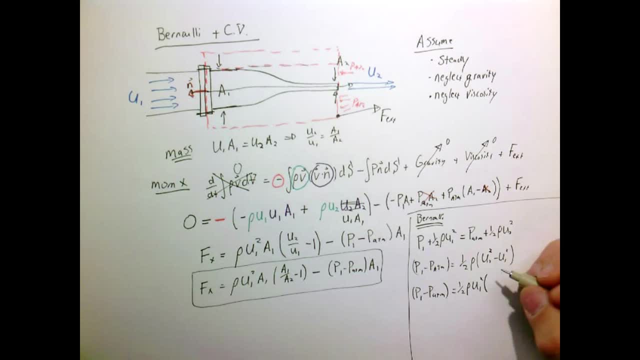 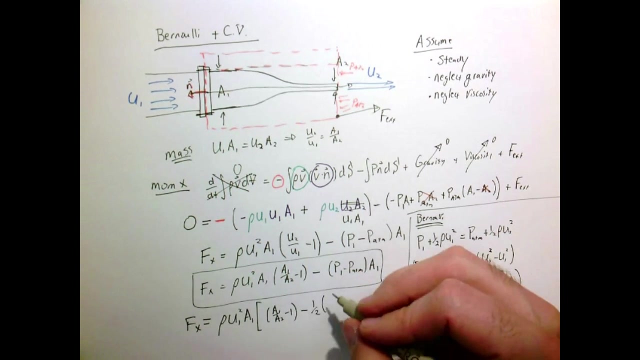 So P1 minus P atmosphere. So now we have a factor of A1 over A2 squared. So let's make this substitution So we get a final estimate of the force to hold this nozzle on in terms of the inlet velocity and purely just the ratio of the area. 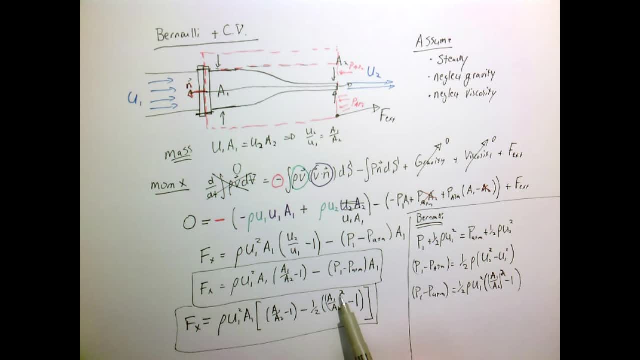 So A1 over A2 minus 1 minus 1 half, A1 over A2 squared minus 1 half, It turns out that if we evaluate this for A1 over A2 being greater than 1, it's always negative, which goes with our intuition. 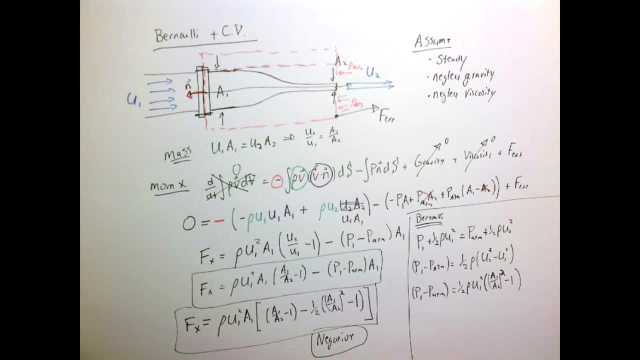 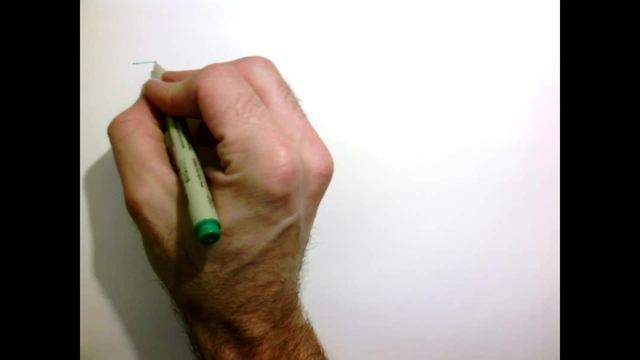 And if we have a hose and we attach a nozzle onto it, it's going to pop off unless we screw it on. OK, let's do one final example where we have gravity in the problem just to do that. So let's do our hose. 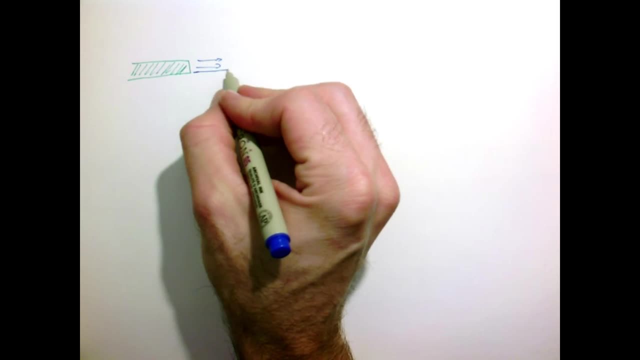 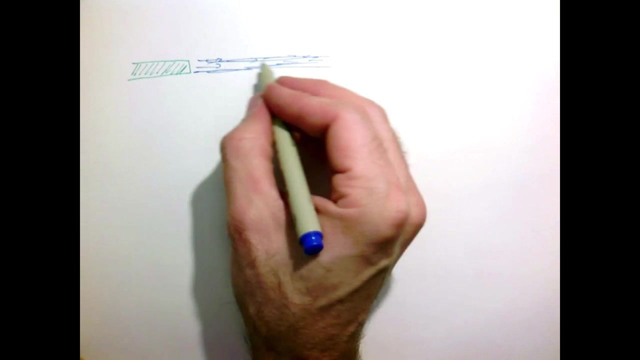 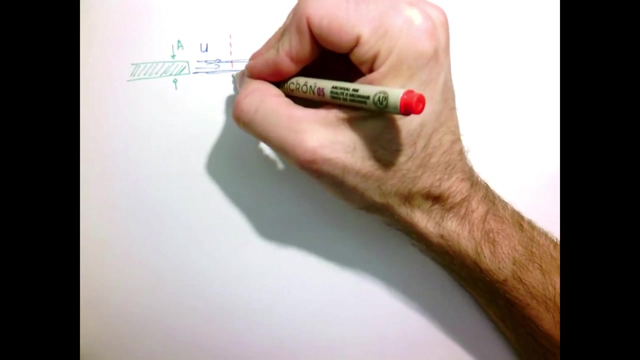 Let's just squirt our jet, All right. All right, So here's my jet out into the air. I'm watering the garden, So here's my jet. It's coming out with velocity. U, Area A. I'll draw a control volume as such. 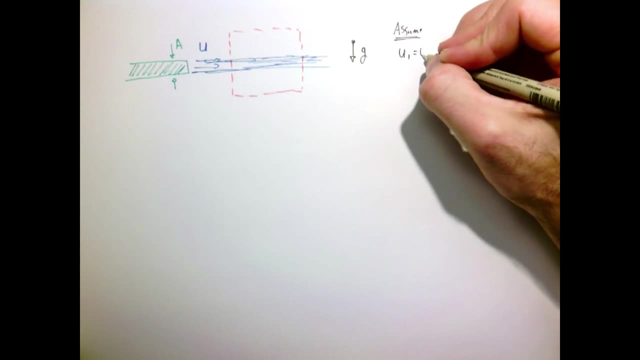 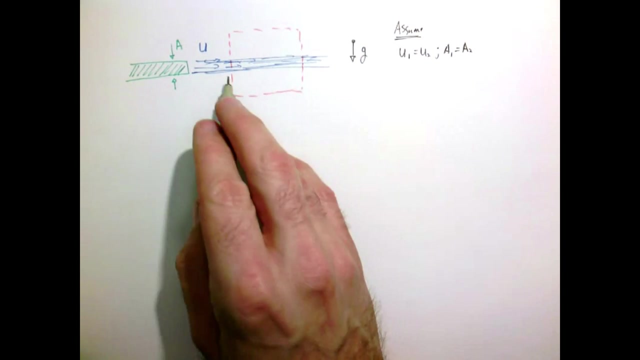 Gravity will point down. So we're just going to assume that the area of the jet doesn't change. so the area here is the same as the area here. Therefore the velocity here and the velocity there will end up being the same. So we're not going to worry about conservation of mass. 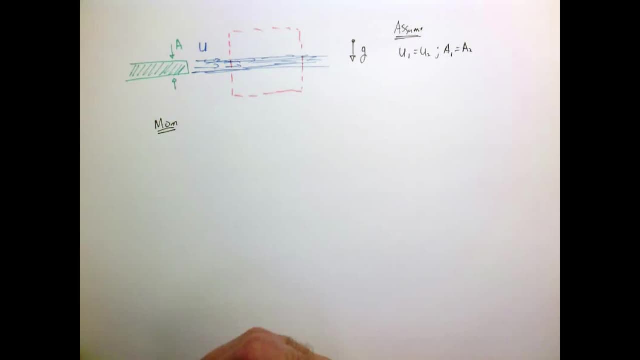 So let's look at conservation of momentum, Let's look in the x direction. So we'll do steady again, So we'll say that's equal to zero. So we have the flux of momentum coming in and out, We have gravity, We have the pressure. 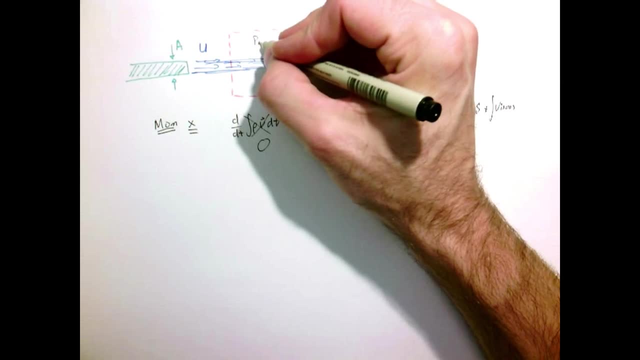 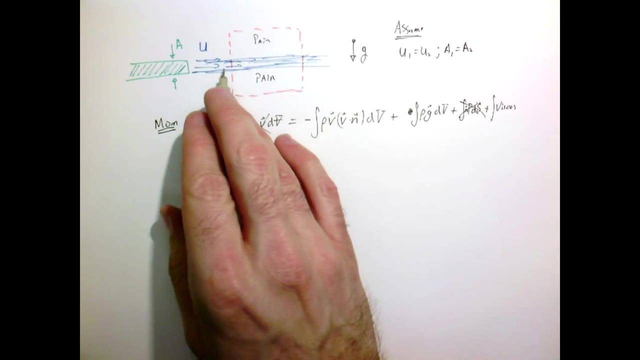 We have the stresses Now as before, with all our free jet problems. since this is p-atmosphere, this is p-atmosphere everywhere, we don't expect there to be any effect of pressure, And since this is a free jet, we really don't expect viscosity to matter here. 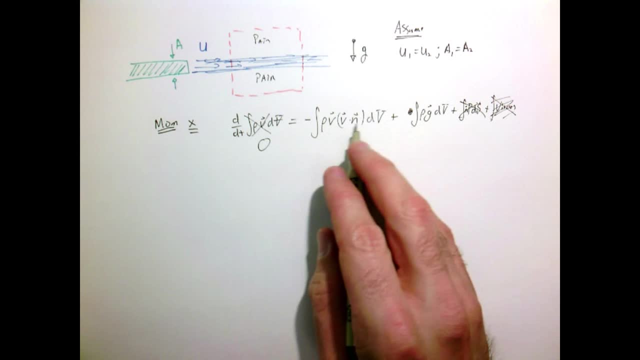 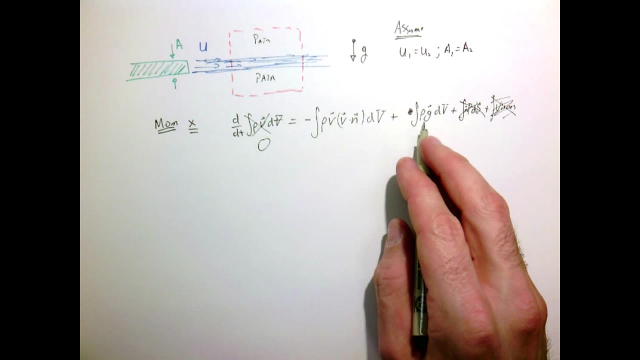 So we're going to cross viscosity out. So our conservation of momentum. we have two components, which is the flux of momentum in and out, and gravity. We look at things in the x direction, There is going to be no gravity, And so we've done this enough before that. I'll just sort of write the terms out. 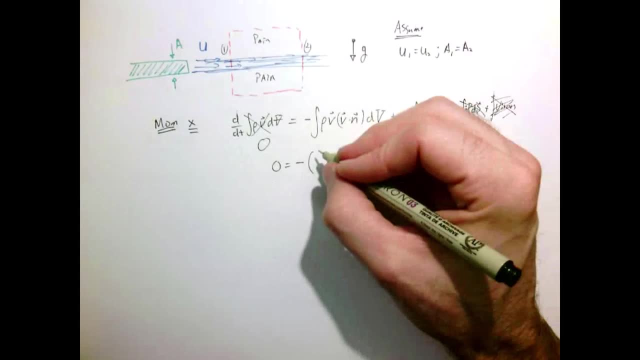 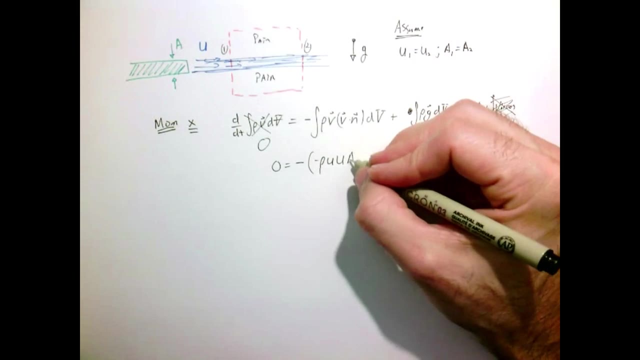 This is surface one. This is surface two. We have a negative sign. We have rho u coming in. We pick up a negative sign. We have u. on the other side We have a And then on the exit we have rho u u a. 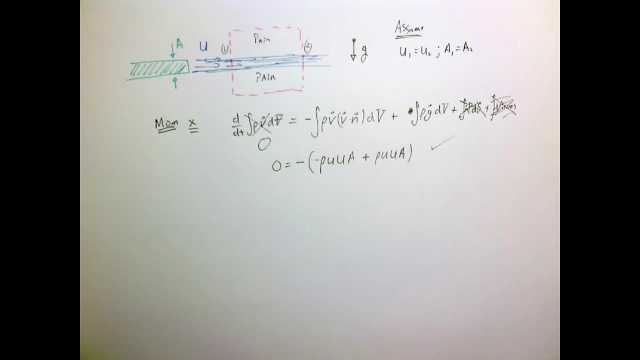 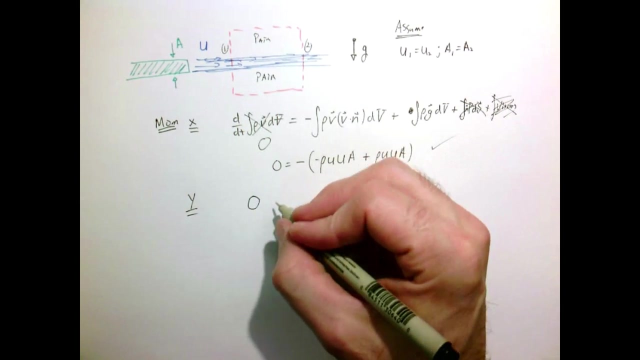 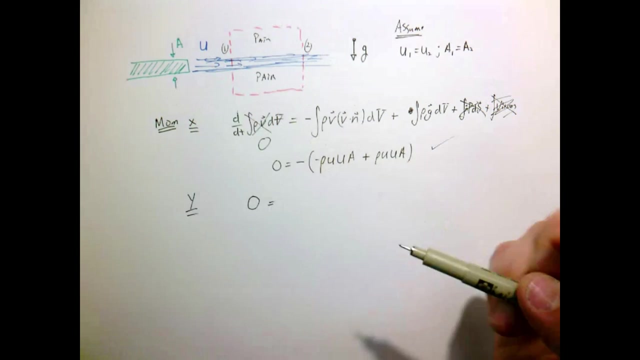 So those cancel. So conservation of momentum: stuff comes in, stuff goes out. Now let's look at the y direction. So this expression still holds. So we have zero. equals Flow is coming in And it's perpendicular, So there's no component. 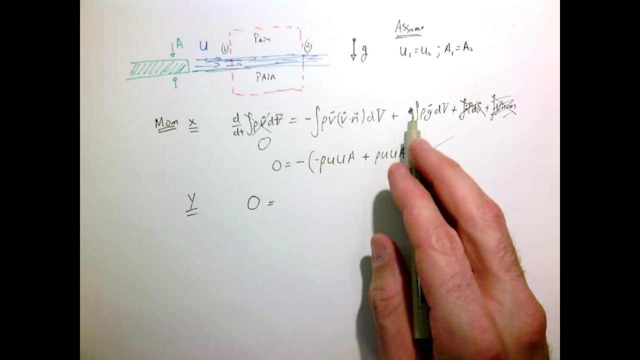 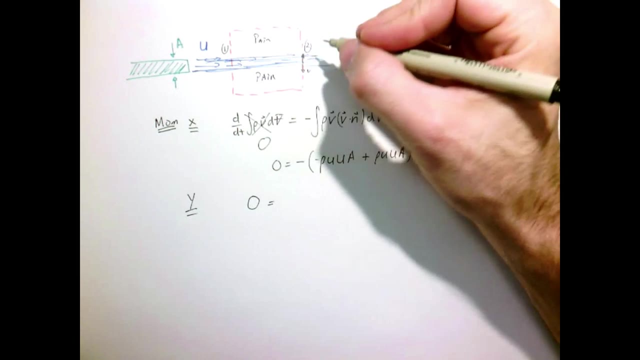 Here, though, something has to happen, because we're going to include gravity. So let's just assume there's a little bit of flow downwards, v. I guess I should assume that it's upward and let the sign sort of work itself out. So we have a negative. 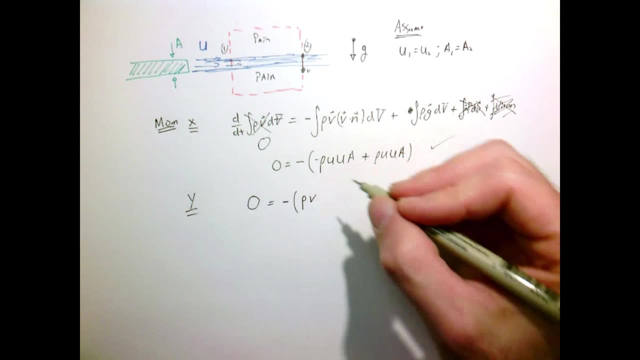 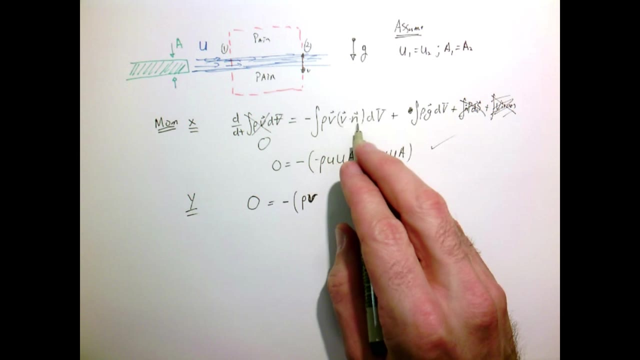 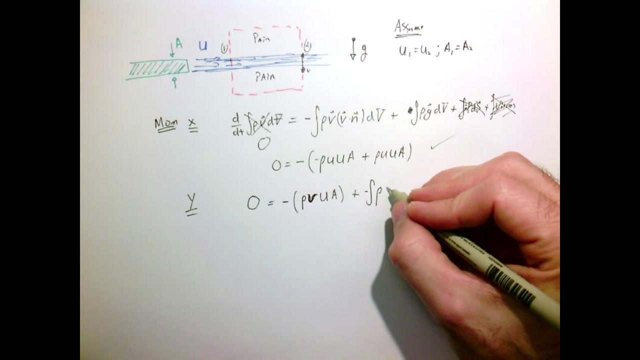 This negative. here We have rho v, So I'll use script v, So the vertical velocity, And then v dot n is the flux of that, leaving that, So that's u times a times the area of the jet, And that has the balance, rho g, which is negative because gravity is pointing downward. 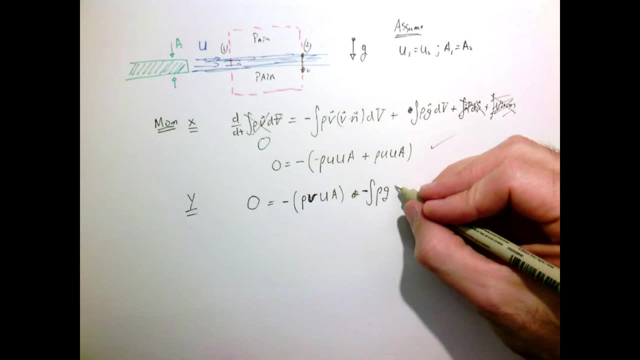 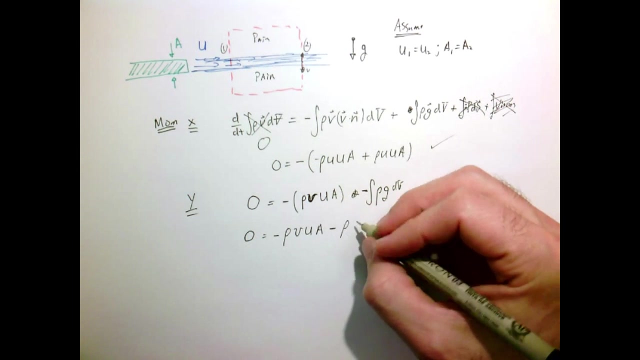 So I'm going to flip that sign to be negative And I need to integrate that over dv. Now the volume of the thing we can just approximate is the area of the jet. Yeah, The length. So this would be zero equals minus rho v u a. 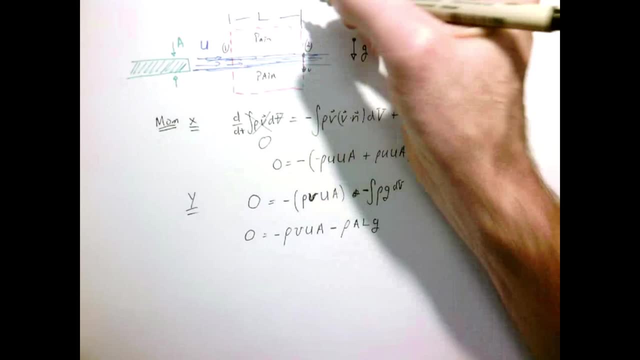 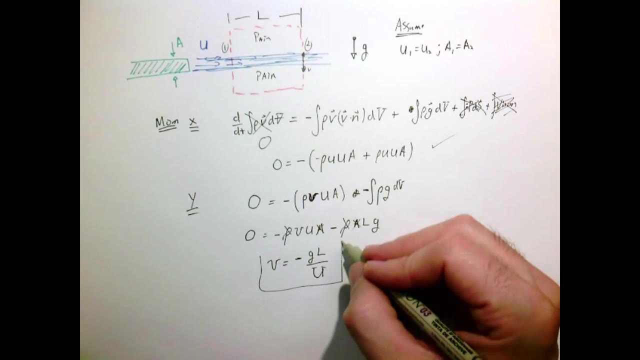 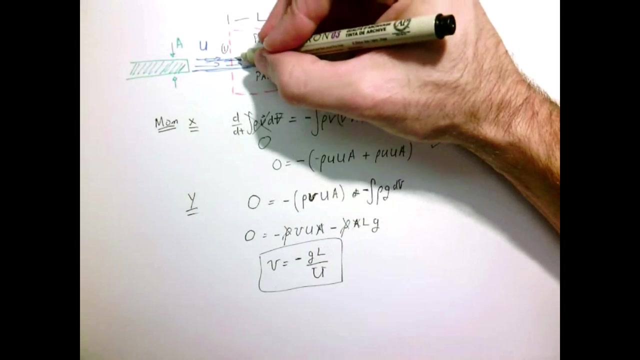 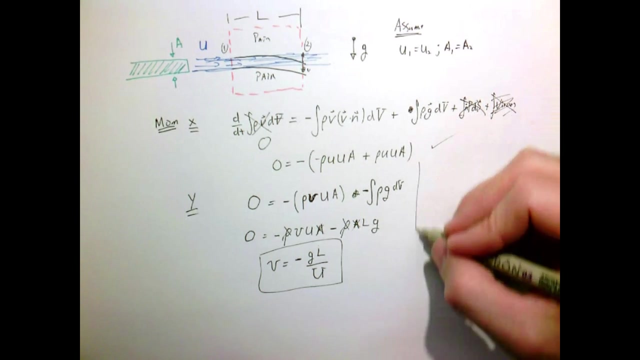 So the area times the length, That's the length of l, So we get the vertical velocity is negative, So it's flowing downwards, is gl over u. So that means that our jet is sagging, Which makes sense. And this also makes sense if we think about just sort of from a particle perspective. 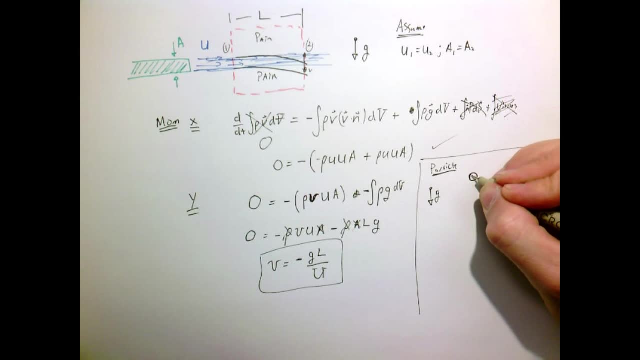 If I have g pointing down and I take something and I drop it, its velocity at any given time is minus g because it's going downwards times the time how long it's been falling for right. So in our case, the time that it's been falling for is this length divided by that velocity. 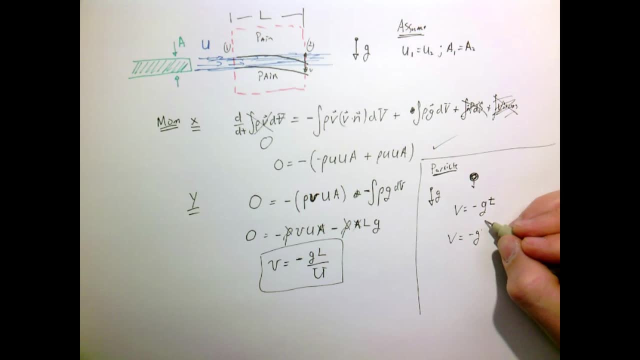 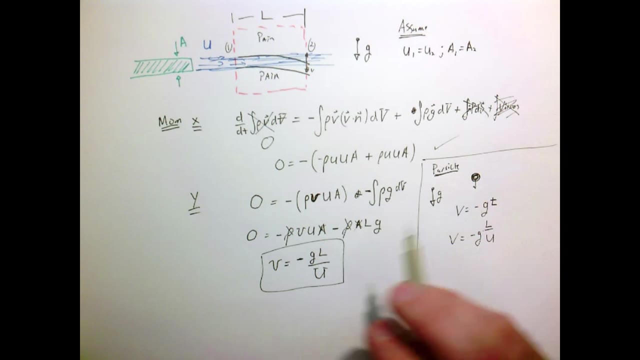 So if I just substitute that in for the time, it's length divided by velocity, So we get the same result. So this is just to show you sort of a simple, sort of trivial example that if we include gravity, yes, things in fact do work out as we would expect.